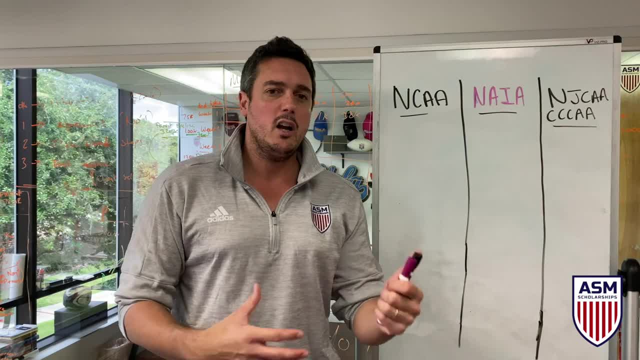 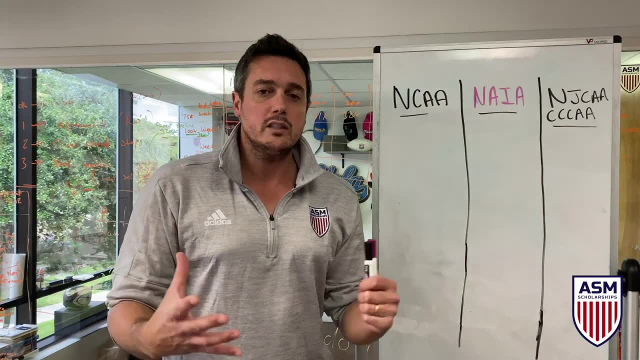 And also what's good about them, what's not so good about them. So I'll kind of go into detail about this. If you've got comments, please leave a comment below. We do love seeing your comments and answering back to them, So these videos are all designed to help you navigate this. culture of ASM. I'm Ernie Els and I represent ASM, So if you've got comments, please leave a comment below. We do love seeing your comments and answering back to them, So these videos are all designed to help you navigate this culture of ASM. So if you've got comments, please leave a comment. 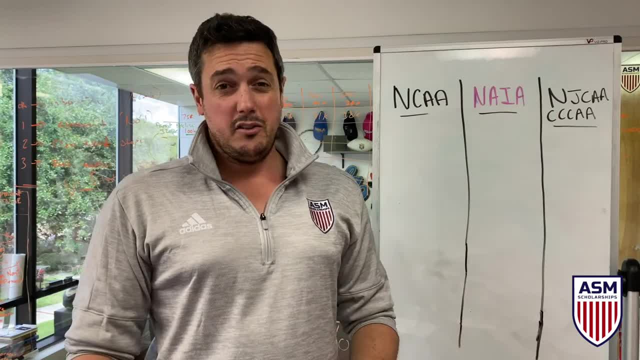 below. We do love seeing your comments and answering back to them. So these videos are all part of an ASM scholarship journey for all of our customers and laughter gratitude all of you guys. Today's video, this week's video, is all about ASM. It's all new to you and you have no idea. 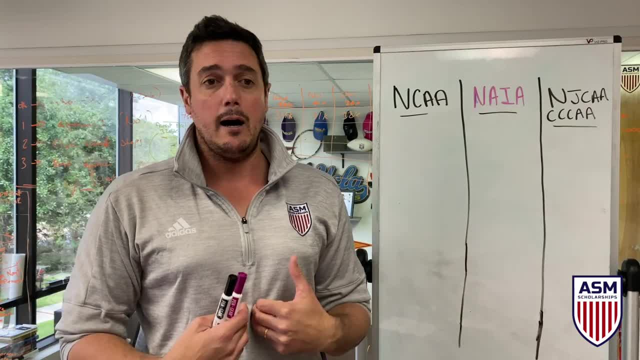 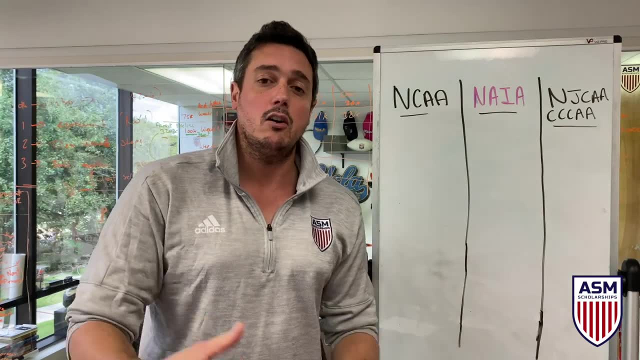 what you're doing. I certainly didn't when I was 16 and had no idea what you're doing. So I'm kind of doing this just to help you guys understand it. and if you are looking for help, you want to get seen and be promoted by us and get someone to see your profile. You can just check out. 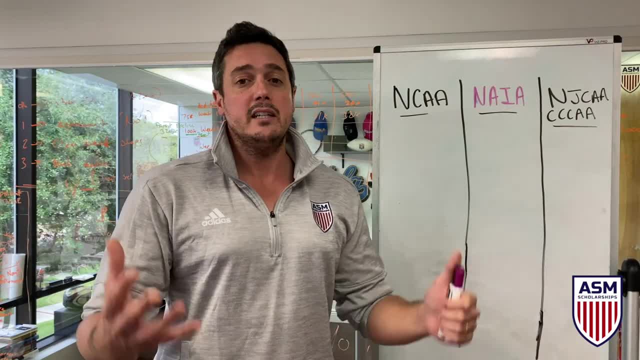 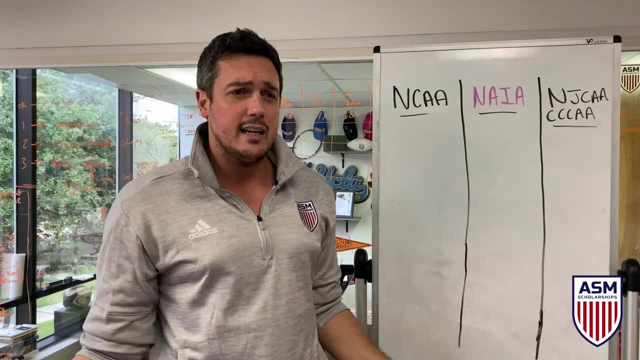 ASMScholarshipscom. You can build a profile there and within a couple of minutes, ourcción director, or ASM college coach, will be looking at your information and contacting you directly. There's a different amount in the whole of the United States. There's different. 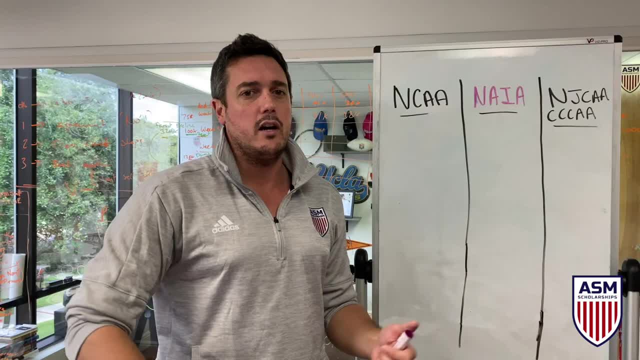 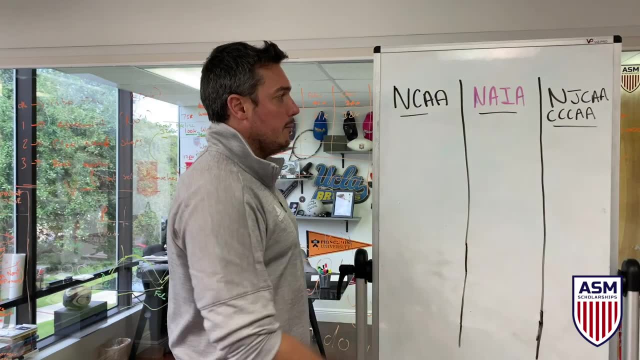 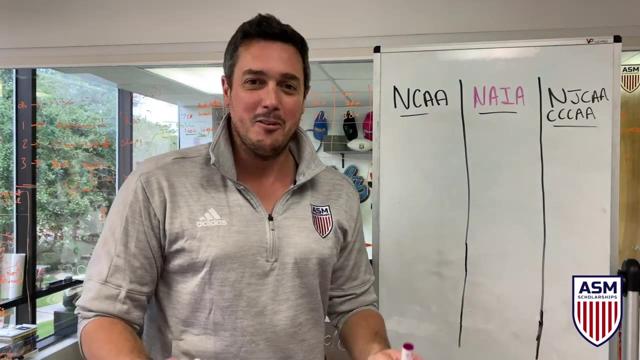 So different associations And the biggest one, the one that's kind of the most on TV for most sports like basketball, football, golf, soccer, all of them really is the NCAA, which stands for the National Collegiate Athletic Association. Didn't have to rehearse that. I've done it for long enough to know it, But it's quite a lot of chunk of work built into one. that's why it's called the NCAA. 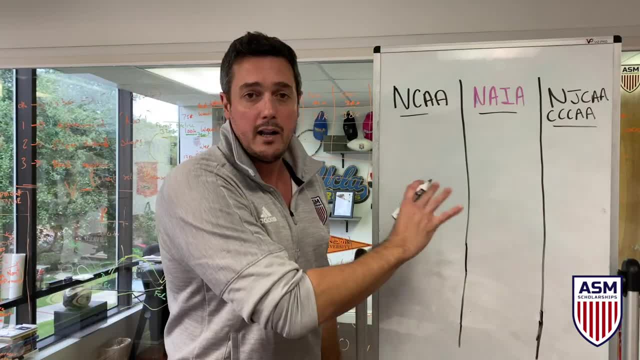 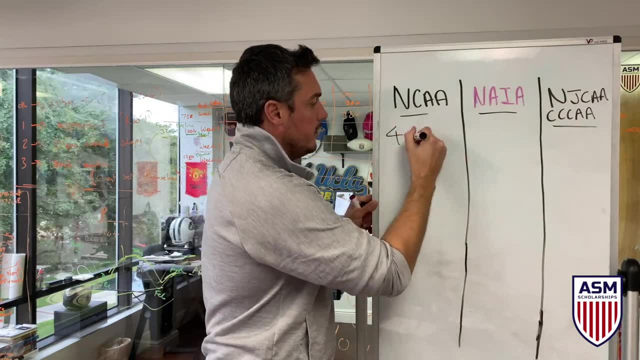 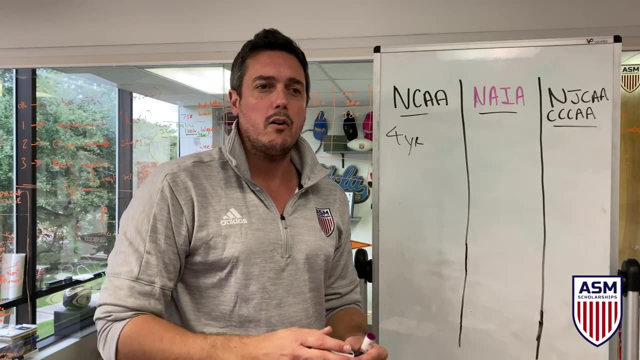 And what the NCAA effectively is. these are, by the way, all universities. We'll get into that. a lot of people think this is not a university, but it is. This is a four-year university. Now, roughly there's about 350 Division I programmes. there's about 1,000 all in all between Division I, Division II, Division III. 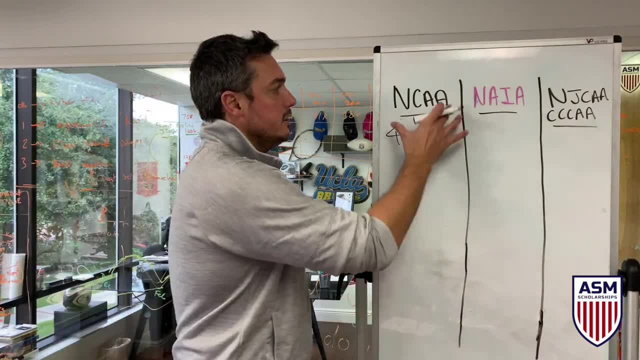 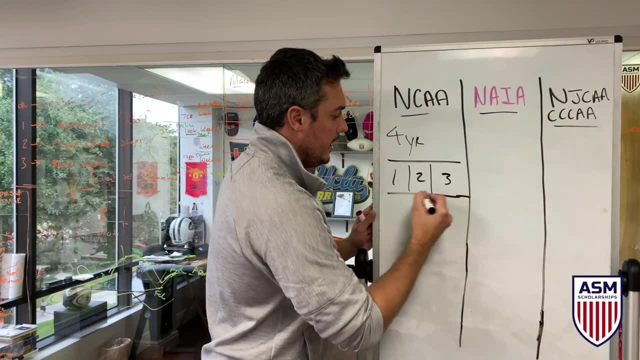 You're probably thinking: whoa, whoa, whoa, Chris, what did you just say? Yeah, so this is the association, but you have three divisions: one, two and three. Okay, Now, typically the best of the best schools for sport. let's take academics out of the equation here. it has nothing to do with academics. 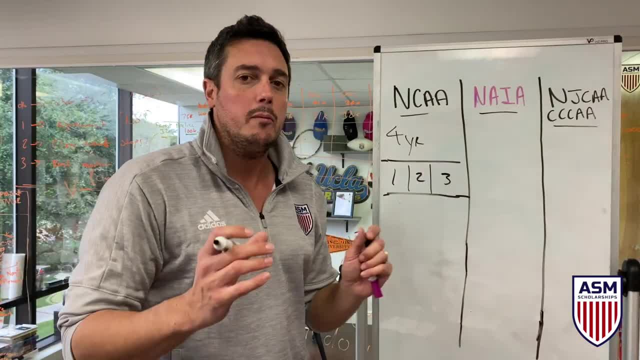 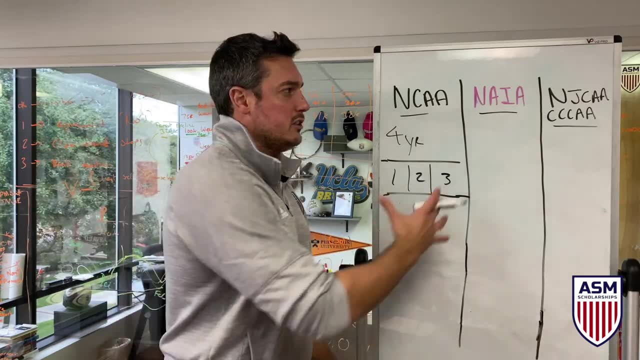 This is all about sport, kind of the money that goes into it. A lot of people think this is automatically the best division because it's Division I, but it's not always. We'll get into that a little bit later in the video: what's the best one for sport and why that is. 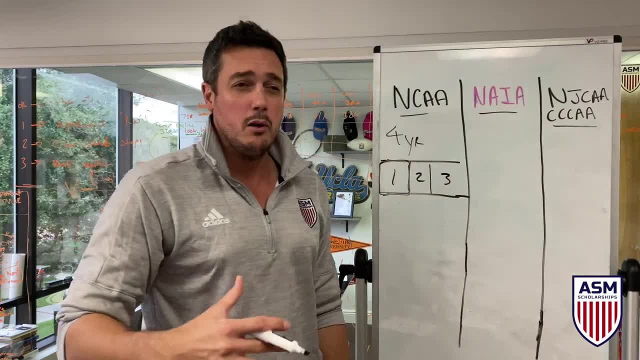 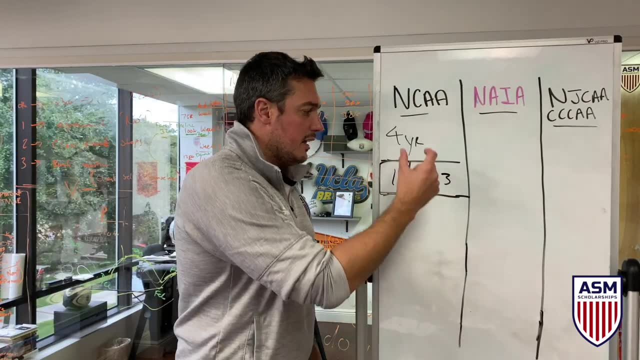 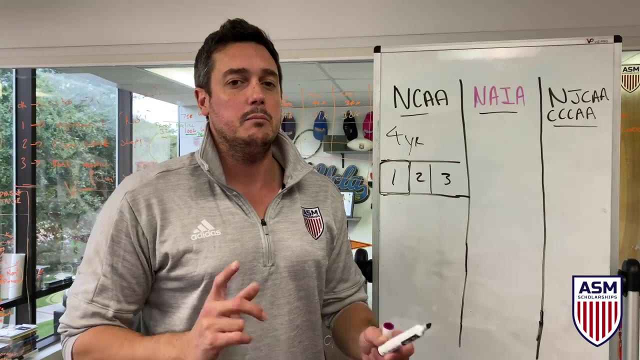 But this one definitely gets the most funding. Division I gets the most funding, which means more scholarship. money is traditionally in Division I universities, Then Division II universities. less funding, Division III: there is no athletic scholarship as of 2020 to give out, but there is academic money, so there's a big difference there. 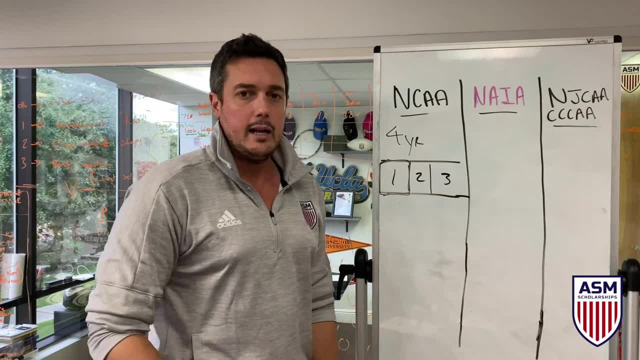 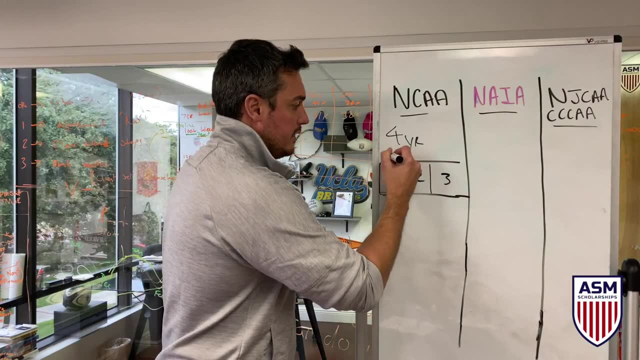 We have other videos explaining that. So you can still go here and play sport, not on a property of sports scholarship, but probably on an academic scholarship. There's also the IVs, which is basically seven schools. That's also part of the NCAA. They typically play in D1, but they also have their own little league. 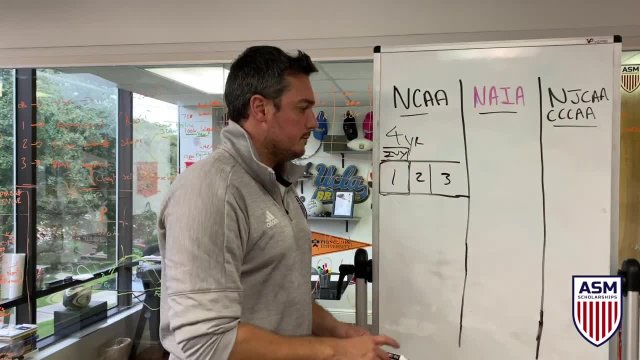 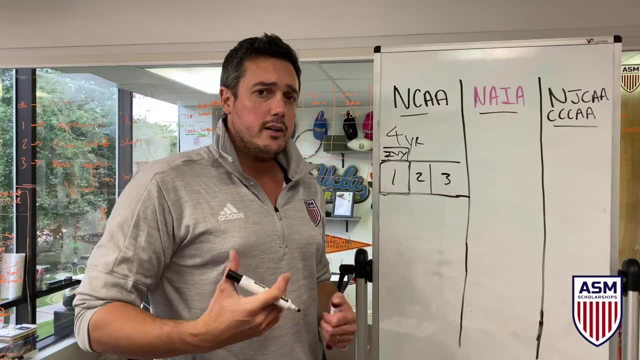 And that's all under the NCAA association. now, to get to a division one, school tip and even division two, you typically going to have to have a couple things. what you're going to need, we're going to need, is to pass high school. that's a must, right? I'm going to pass. 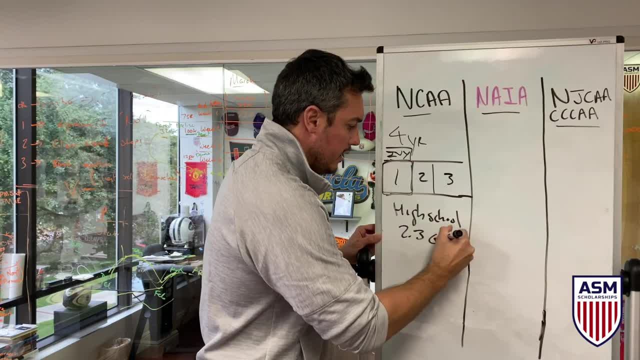 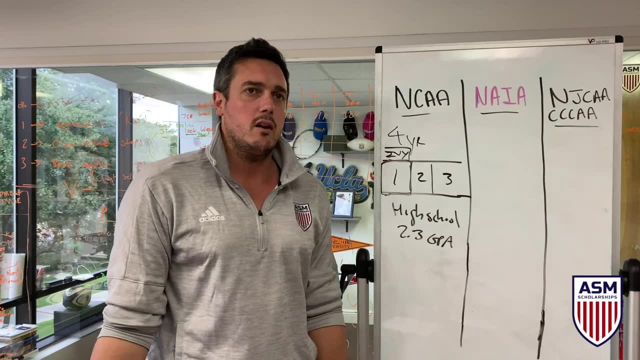 high school typically at least a 2.3 GPA. so overseas, like where I'm from, England, it's like at least a C grade across the spectrum. if you're in South Africa, across Africa it's like about a 70, matric 65, the very lowest about 70. 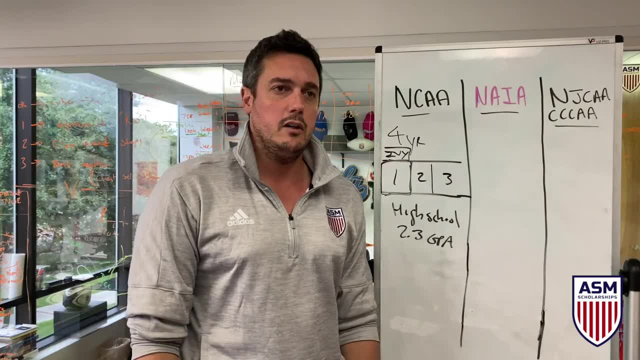 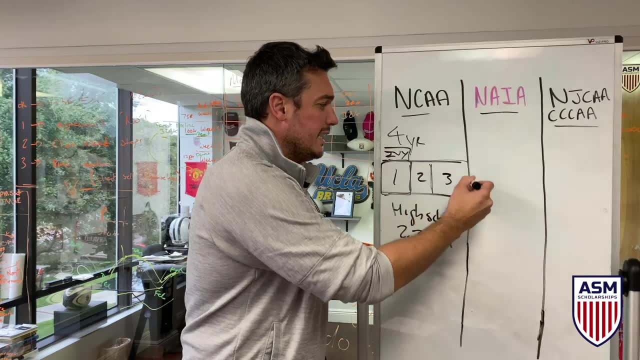 basically just pass high school, right, don't if you. if you're getting D's and E's, I've got another solution for you. if you're struggling at school, you might struggle with one of these divisions, especially division three, because they tend to be better academic programs. so division one, division two is you know. 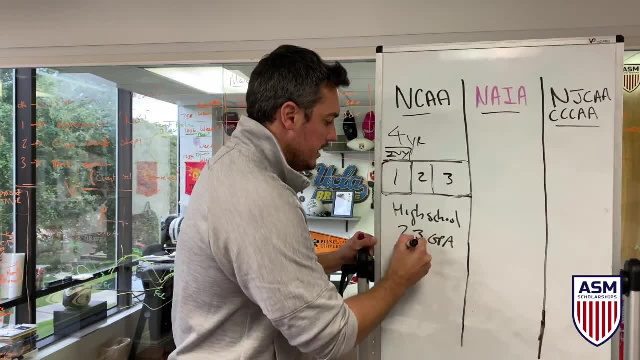 get that. yeah, SAT wise. the minimum you're going to need is a 960 recommended a thousand plus on the SAT. TOEFL is really good, so you're going to need to pass high school. you're going to need to get that. yeah, SAT wise. the minimum you're going to need is 960- recommended a. 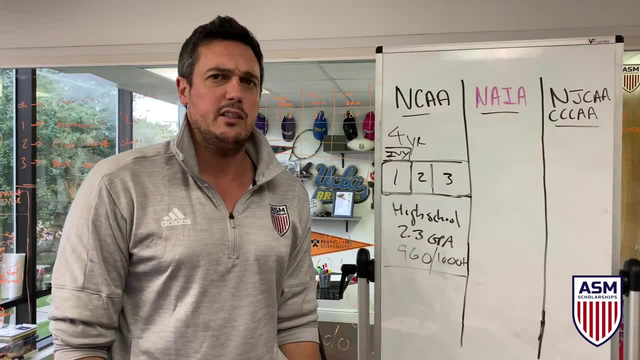 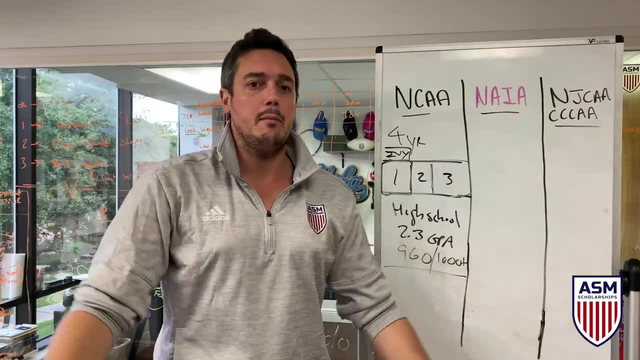 well, you've got to just at least pass the TOEFL. for most institutions I think that's around 70 points now, 65, 70 points on the TOEFL exam. so that's what you need academically now. sport wise, that's a whole different ballgame, I mean. 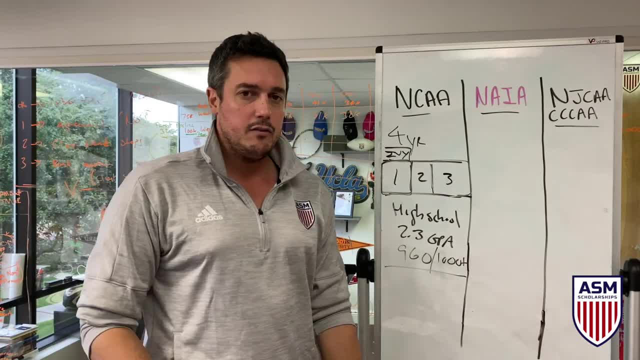 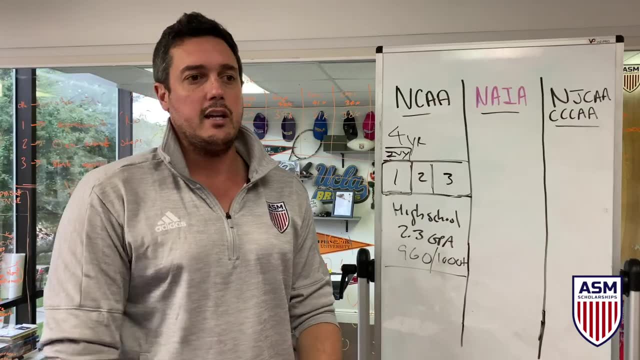 that varies a lot from program to program, but typically, if you're looking to get a full ride scholarship, which most of you guys are, you're going for the division one school. these are schools like UCLA's, Florida State's, Alabama, Texas A&M, Stanford, right, Berkeley. these are typically division. one programs. typically for those programs you've got to start this process early to get advantage, because they look for players super early and if you haven't gone into one of these division one programs by the time you're 16 and a half years old to 17, you need to start wanting panic. but the chance of 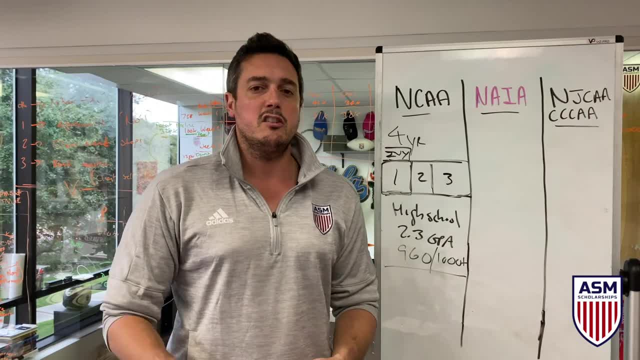 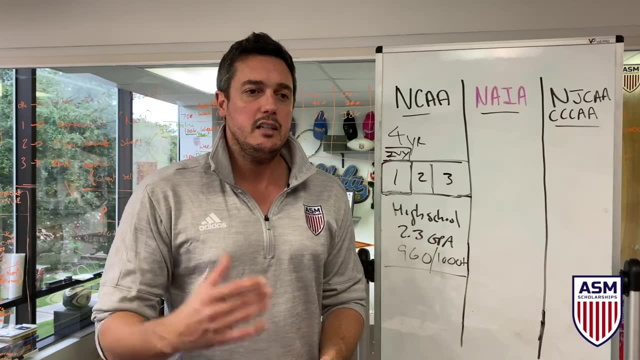 you getting a full ride are less and less. unless you're playing sports like basketball, American football, they tend to recruit a little bit later, even soccer a little bit later. but yeah, you need to be ahead of the game for division one and you need to be in more the top echelon of your sports. what I mean by that? 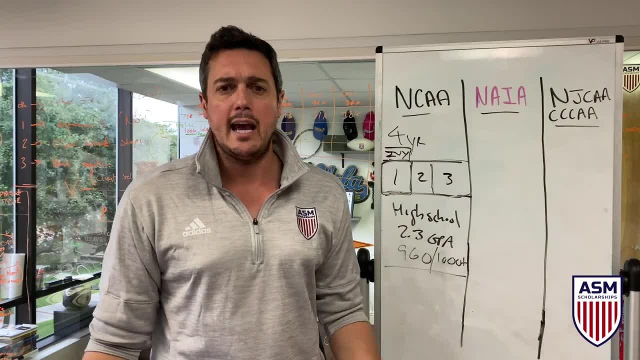 well. if you're playing soccer, you should be playing for a very good youth academy program. if you're playing golf, you should have at least a WAGA ranking of 2,000 or better. if you're a tennis player, you should be a UTR of at least. 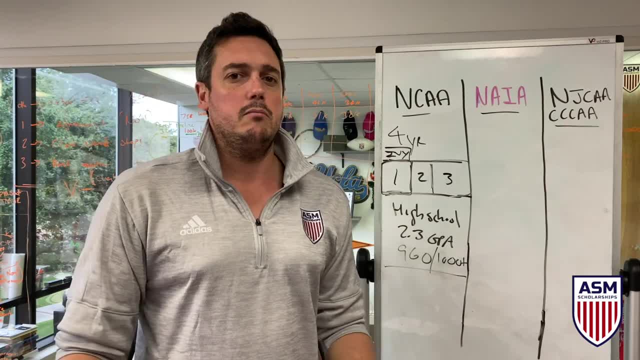 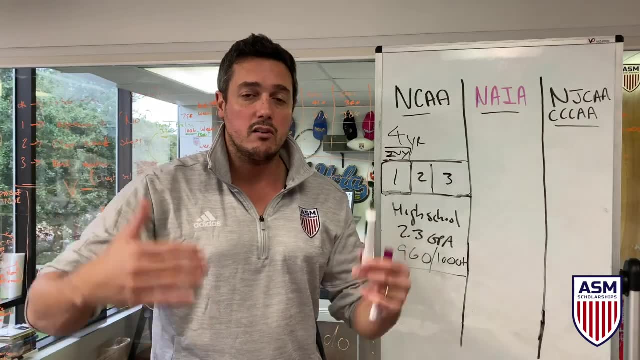 ten and a half eleven up. you just got to be at the pinnacle of your sport, for as an amateur you need to be very, very good, especially for the top NCAA division one program. so there are ones that are ranked less than a hundred, like sorry, above hundred, like two hundred three hundred. that's different. you've got more of a. 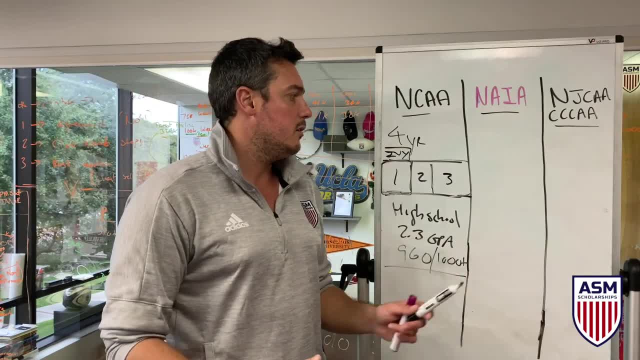 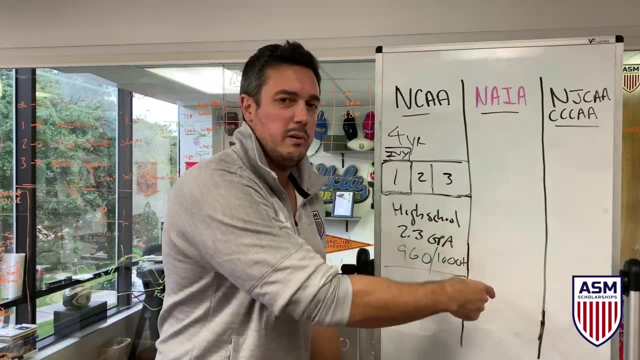 chance getting into those programs and we'll get into that. that kind of goes into that in D2, the top division two programs are just as good as division one programs and I'll explain that after we've done this bit, like in like a couple of minutes time. 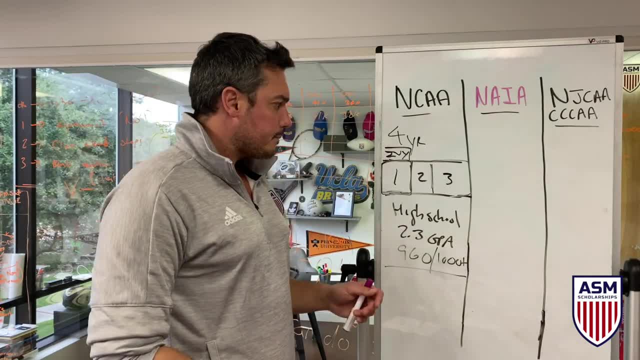 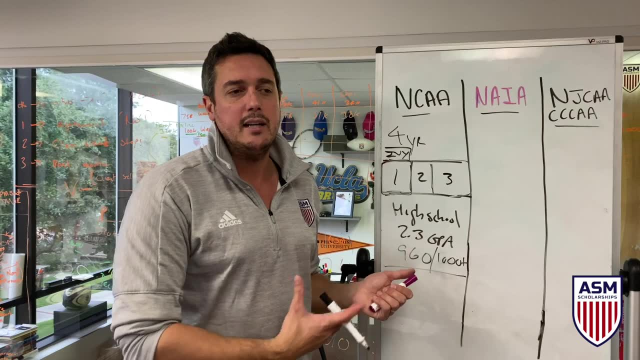 all right. so that's kind of minimum sports stuff. you need full year programs, fully funded, where you get everything paid for, the full ride really, where most people that come to us want to end up. and especially- I'll be honest with you- you want to be a pro athlete. if that's the goal, division one will give you. 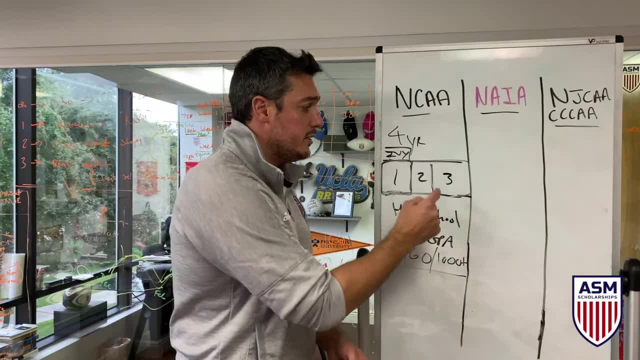 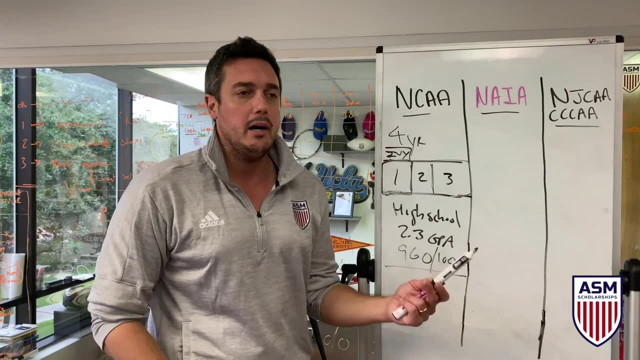 probably the best opportunities for that, especially the drafts. you can do division two, especially the top range. I wouldn't count that out. but if you're looking to be a pro division three, it's possible. but your percentages go up if you're in D1. so that's kind of where I go. now NIA: again. it is a 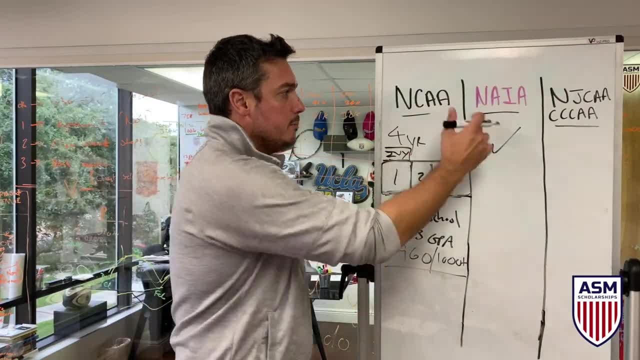 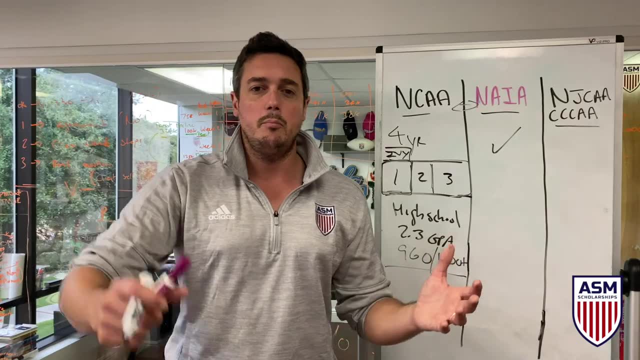 four-year program, same as NCAA. these are basically competitors, right, it's almost like where I'm from England. we've got the Premiership, that's one soccer league, and then you've got the Bundesliga in Germany, then you've got La Liga, right, it's the same kind of thing. they're just like competitors. they just these guys. 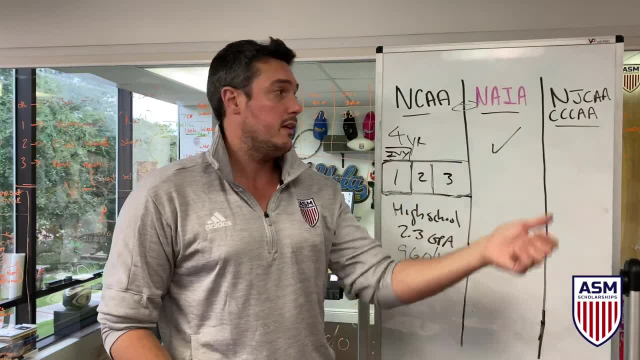 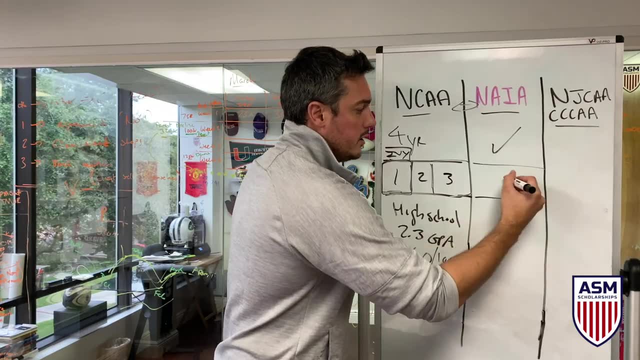 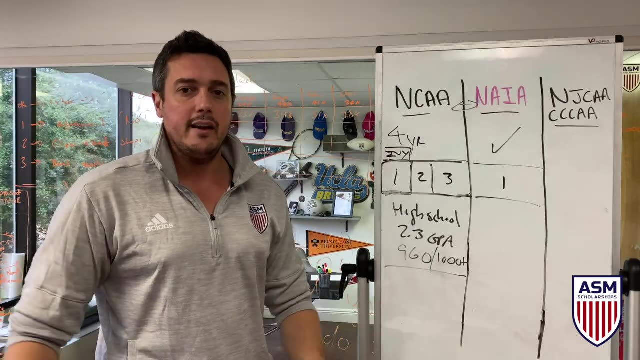 actually start the whole college sports first with basketball, and then these guys came along and did the same thing. so there's two associations. typically there's less funding. they only have one division across the whole spectrum. typically there's less scholarships available, but they are still there. they. 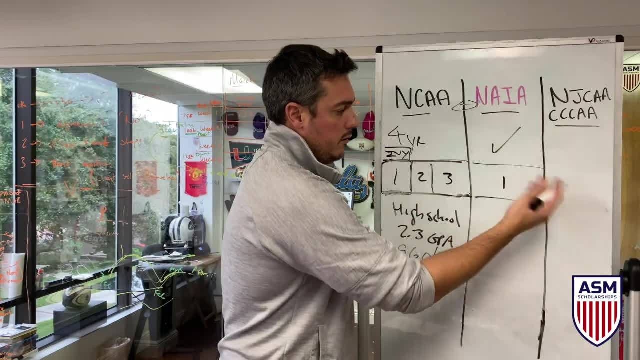 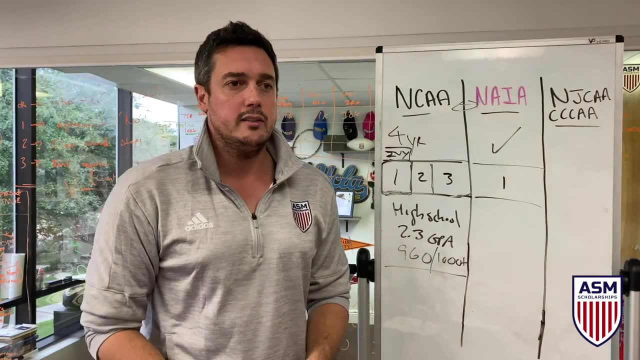 are full rides and at the top level of these, so their universities is very high standard. they tend to be smaller universities as well. when I say small, they're still like you know, 20, 30, 000 some of the programs. some of these programs are like 60, 000, like. 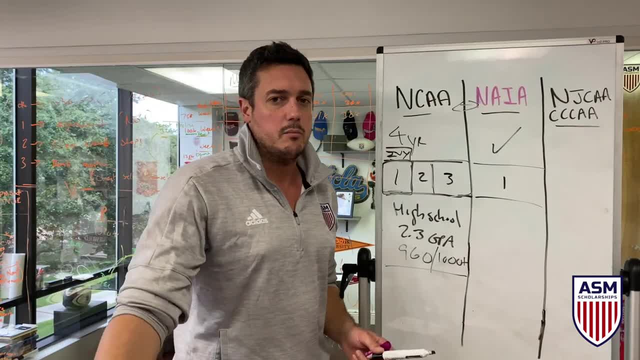 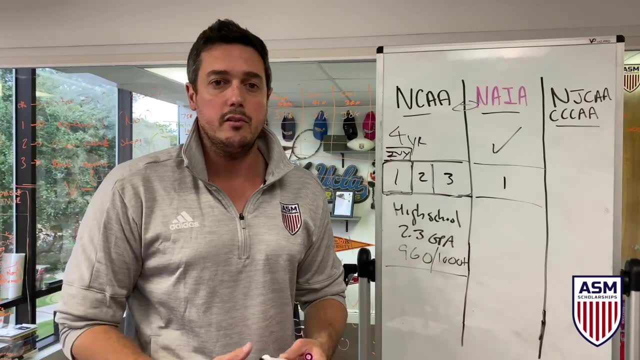 50 to 60 000 students say it depends the program, but they tend to be. if you want to, you know, not have to travel as much of the University and take bus rides and get across campus like these are better places to go. they're the. 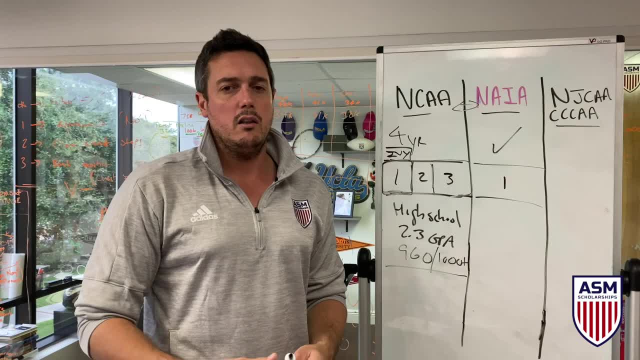 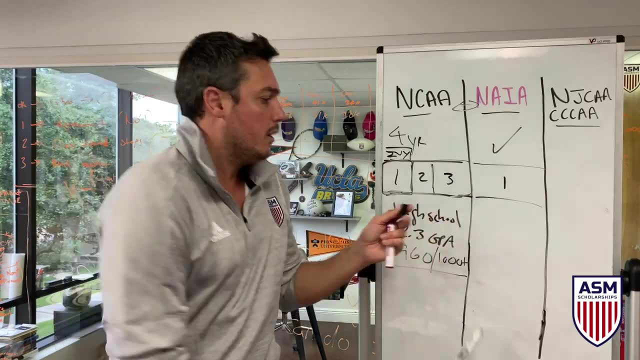 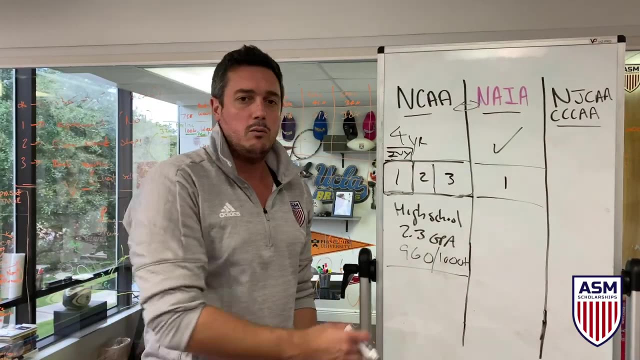 nicer campuses and normally private schools. lots of money's chucked into them. they're very nice places to be. I definitely recommend any NIA program over D1 or D2 program in the location you don't want to be at. if you go to top D1 program, great location, so everything you want, fantastic. but again these go by. 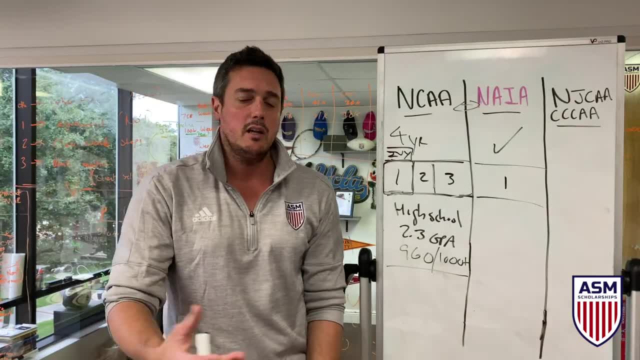 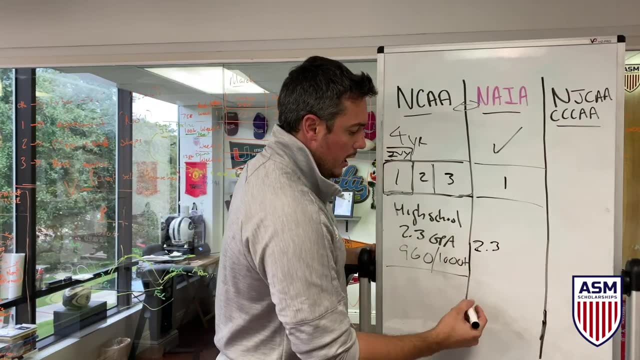 case by case. you really got to think about what are you trying to get out? the experience academically very good as well. again, you're going to need a 2.3 to qualify to get a minimum. you're also going to need the same thing here, right? 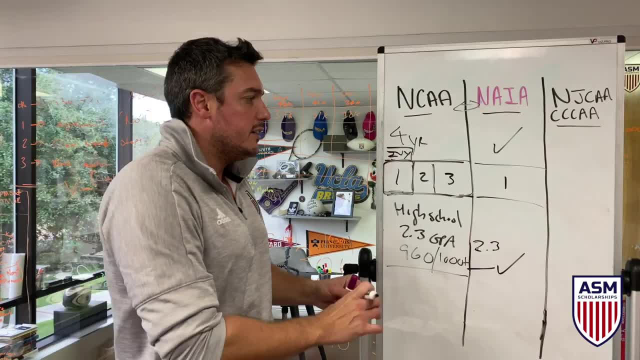 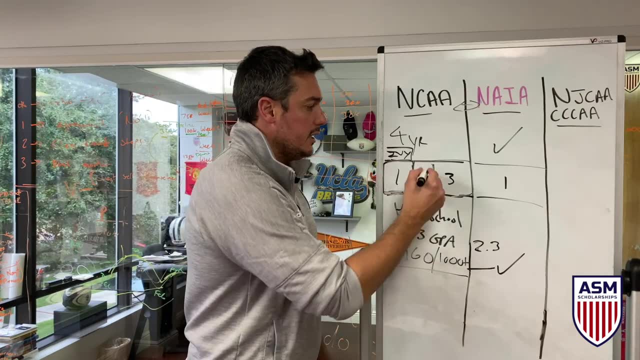 960 1000 to qualify again. they're very similar in terms of qualifications. what you need sport wise don't have to be as good like as a D1 level, but kind of D2 going to be the same kind of standard. that's the best way to describe this now. 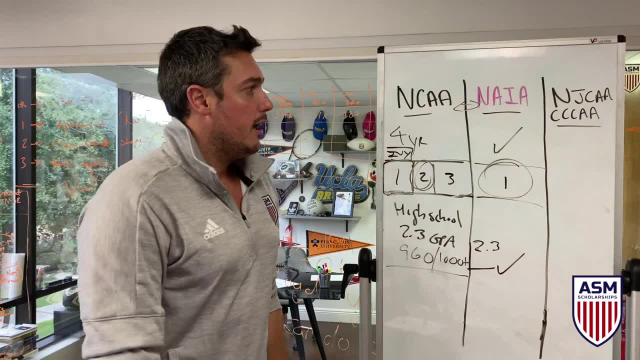 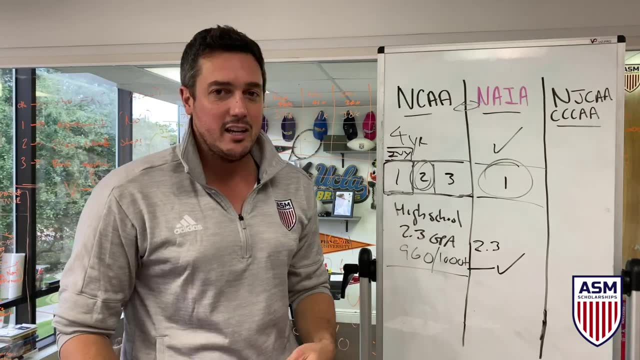 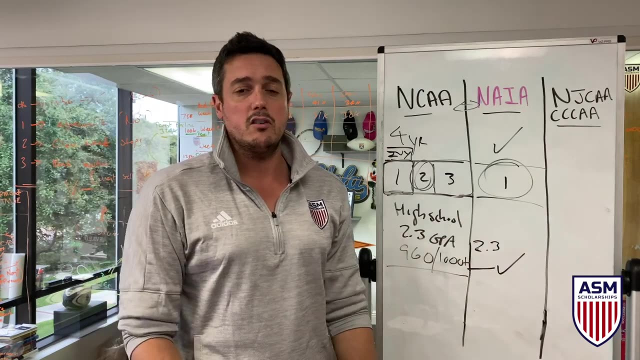 this one, the NJCAA, and the CCAA, basically National Junior College, National Junior College Athletic Association. the other ones, the California Community College Athletic Association. this now a lot of people think this is not the best place to go. I shouldn't go here and this is my. 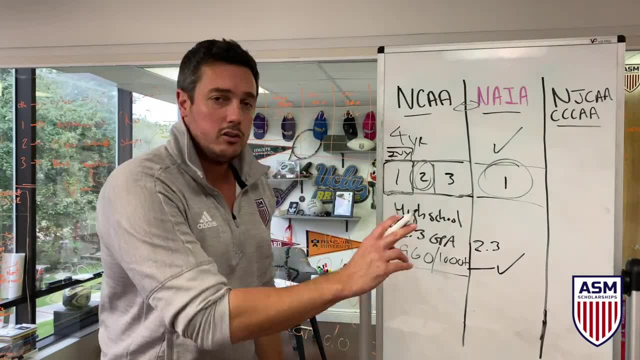 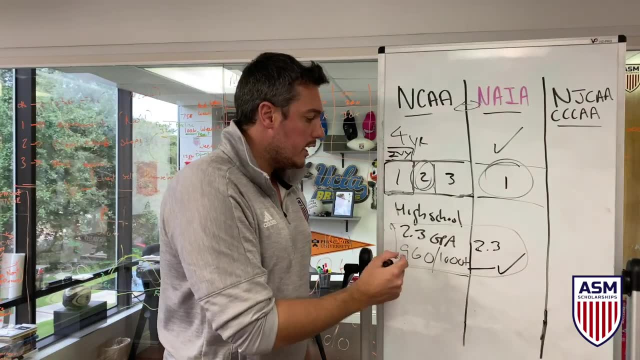 recommendation if you are failing it. there's two reasons why you go to junior college right. number one: you're not going to be able to go to a junior college. number one: you're not going to be able to go to a junior college, right. number one. reason one here: you can't do this right. you're unable to pass your SATs. you're. 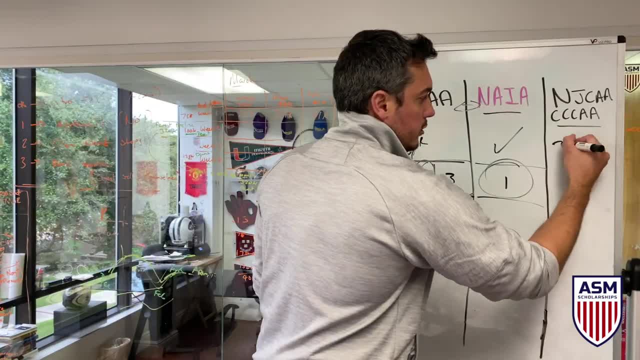 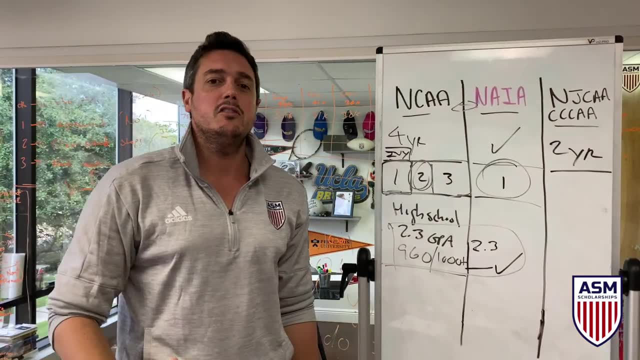 unable to get at least a C grade average. so boom, these are two year schools. by the way, two year universities, they aren't universities. in America. we say college a lot. it confuses people from overseas. that is university in America. so you could say: here, you know, I went to D1, I went to 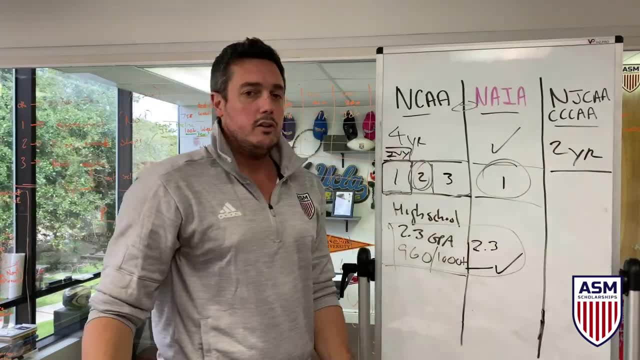 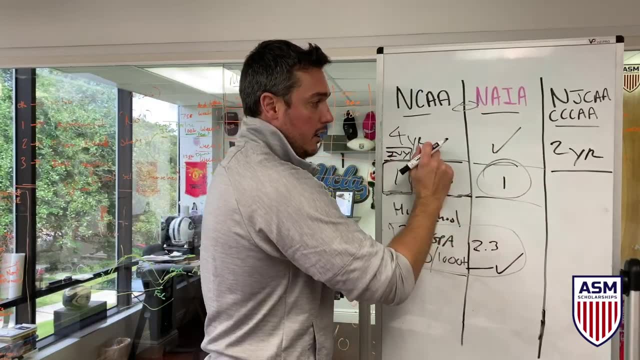 college. well, it's the same thing as going to college here. it's just two years. so you do the first part of your degree and then you transfer everything to one of these two programs. you go here first, you come either here, or you come here after two. 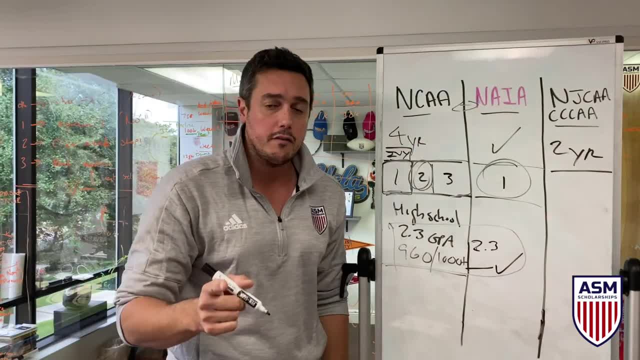 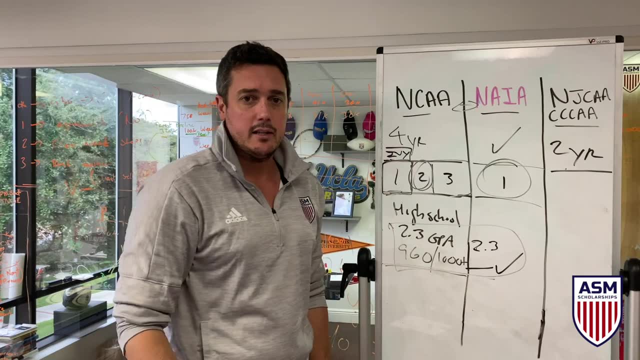 years. you can do one year only if you were a qualifier for one of these programs academically. so, as I said before here, if you didn't have this, you'd go into the academics. but some people have this and they still go to a junior college. why? because they have goals of getting to one of the top. 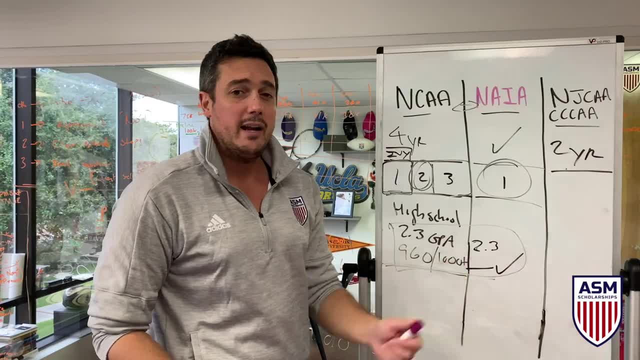 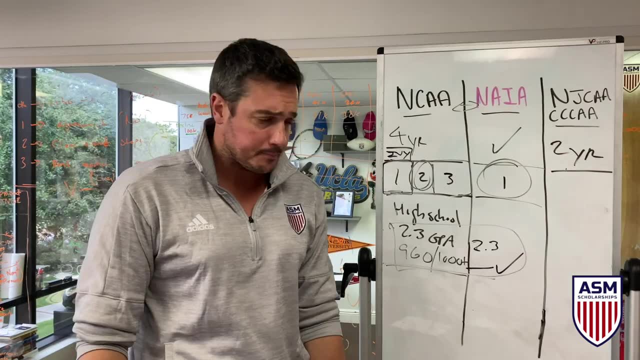 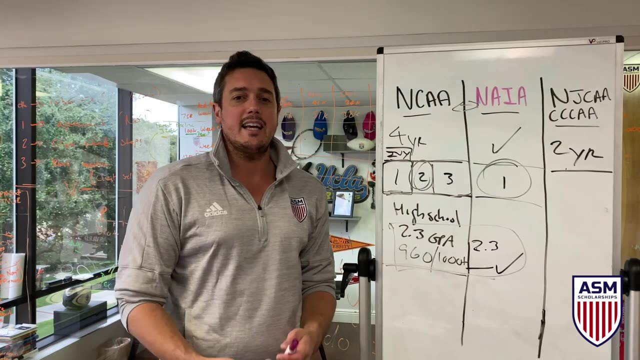 division one programs or a top division two program or even a top NIA program, and they came to the process too late so it wasn't enough scholarship money to get into all these programs. so what you do, and if you have, if you got Netflix, I seriously recommend watching like last chance you. that will give you an idea to how competitive the top of the top junior colleges are and you can get scholarships. you go there there for two years, you work on your level and you're going to transfer here or transfer here after two years. if you're a good athlete, you'll get picked up. we actually help our athletes with the transfers as well. 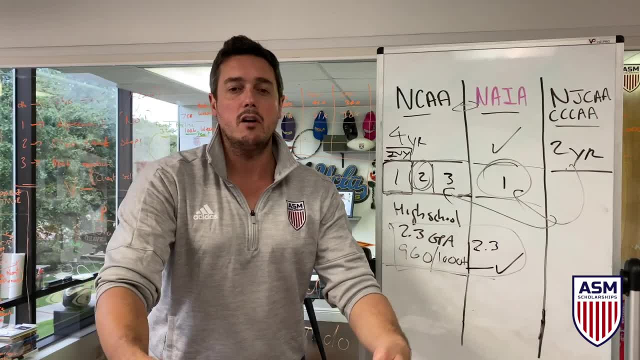 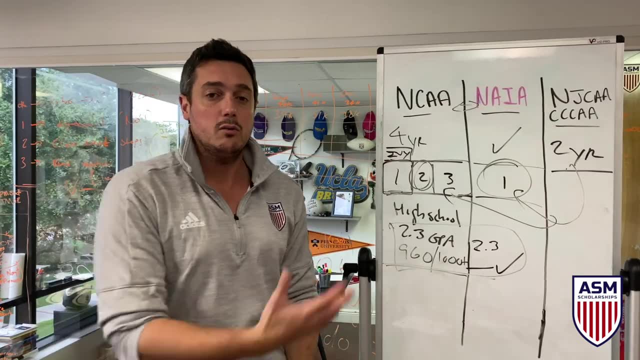 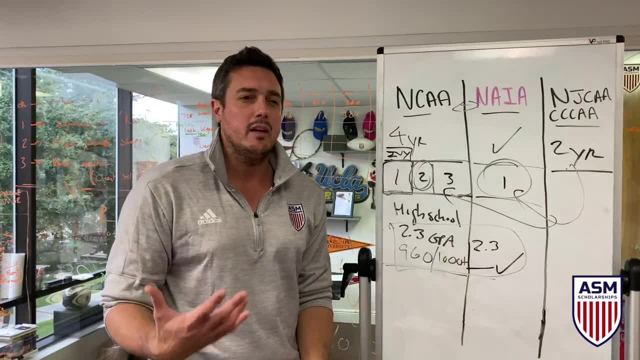 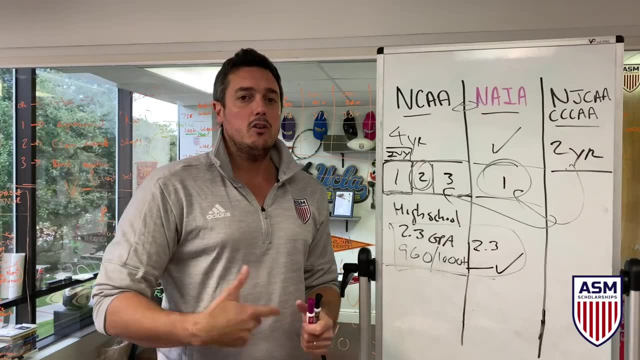 transfer. I left this process too late. I need to. I know I'm good enough to get into these top programs. I'm going to go junior college first and transfer. some of you might be thinking why I'm not just taking gap year. yes, you could do that. you could take one year of a gap year, but there's no guarantee that you'll. 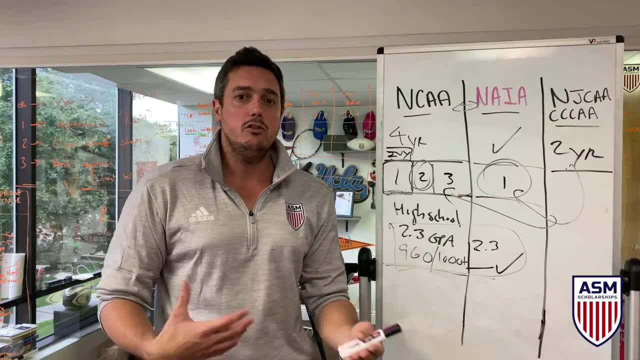 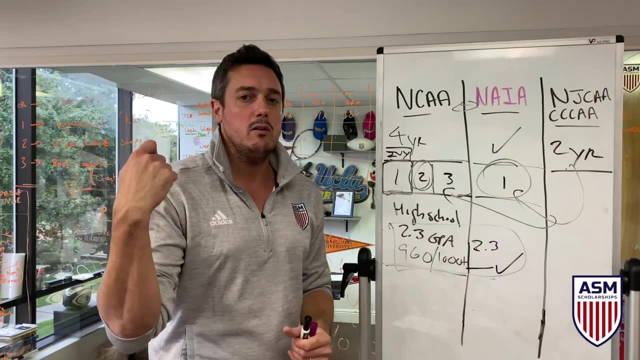 then still get in the good thing with junior colleges. you're in the states, you're beginning your education and coaches at the division one, division two level at North in the States. it gives them more peace of mind knowing that you're going to be worth that investment than never seeing you apply, say, overseas. they just don't know how much you're. 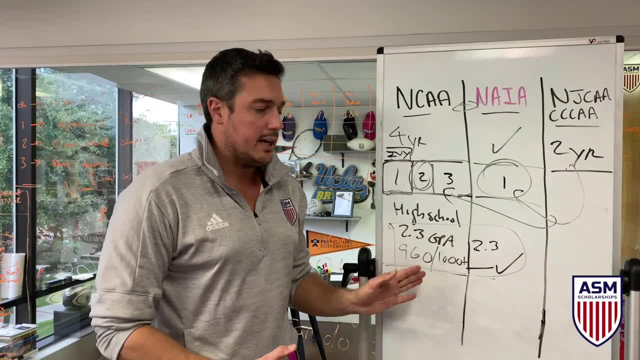 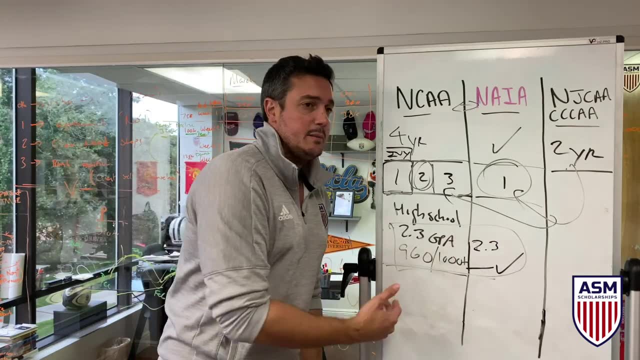 improving by so. I'd always do this. if you're failing academics, it's your only way in. and if you've left this process too late, or maybe your English is like you've passed academics but you feel like your English is like not at the best right because you are going to do a degree in. 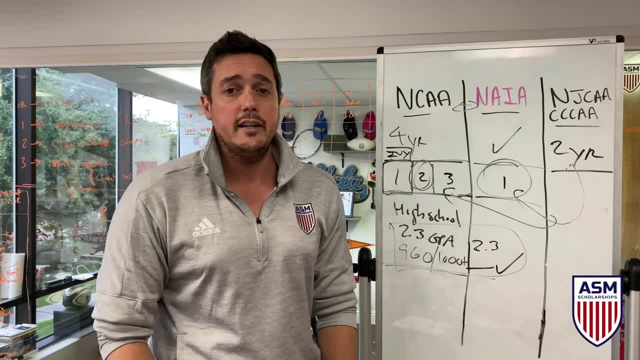 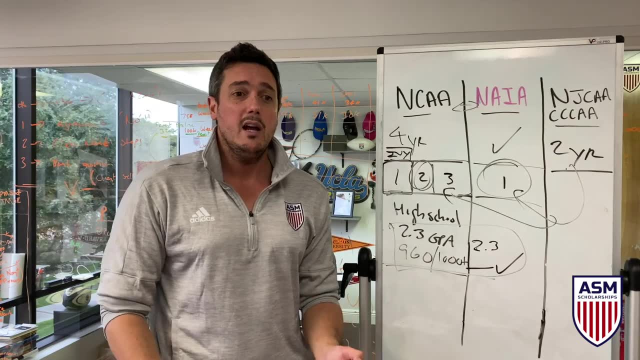 English. this is a great place to start to get used to studying English more full-time in a degree capacity, and then you can transfer your last two years. so it's not so like crazy all at once. right, because, remember, this is college sports. it's still university in sports, hence it's called college. 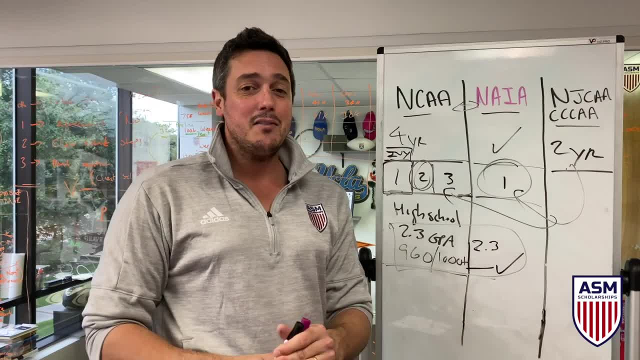 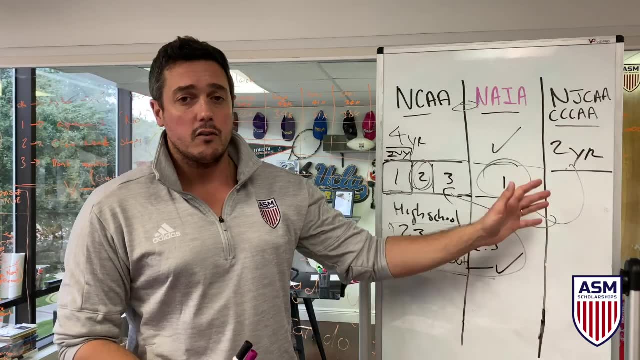 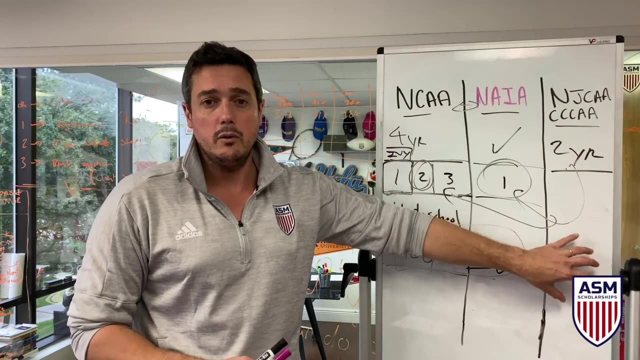 sports, not just sports, right, so you're going to have to study. if you don't feel like you're strong enough in your English to study English, then maybe JC is a better option, first for a year or two years and then you transfer. pretty much. I love this place if you, if you like school you struggle with. 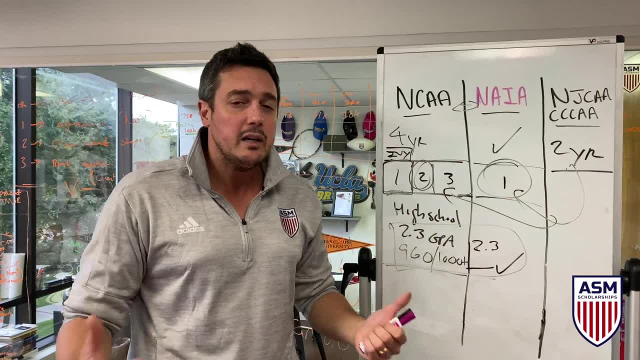 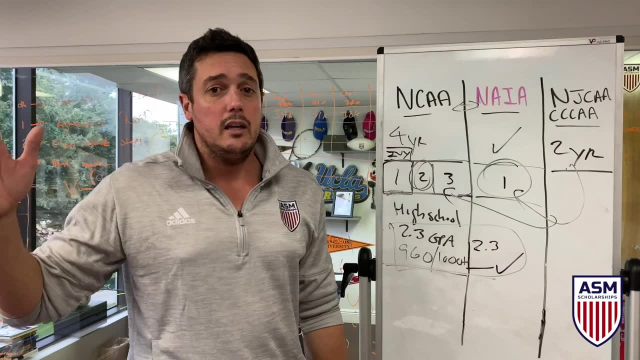 it's one of the most easy places to get used to it. it's like being back at high school, but a bit more tougher education, and then you're just going to end up on a top program if you don't know. now here's a risk if you don't. 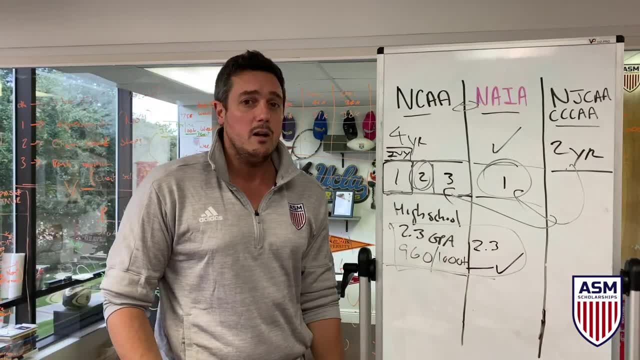 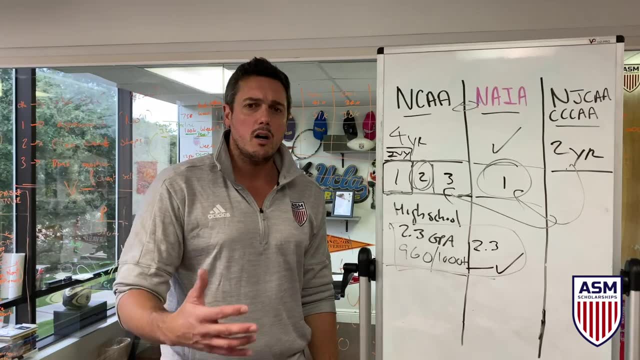 do well and you start over here and you don't play well, you don't get the results. you will find it really hard to transfer. that is I'm just going to be honest with you. it's not guaranteed, but if you do come out, you work hard, you will end up in a better program than if you started the process. 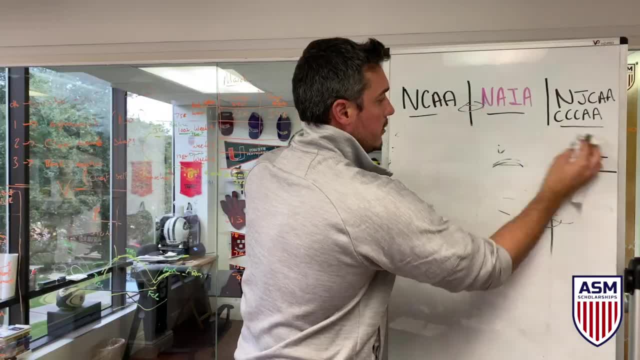 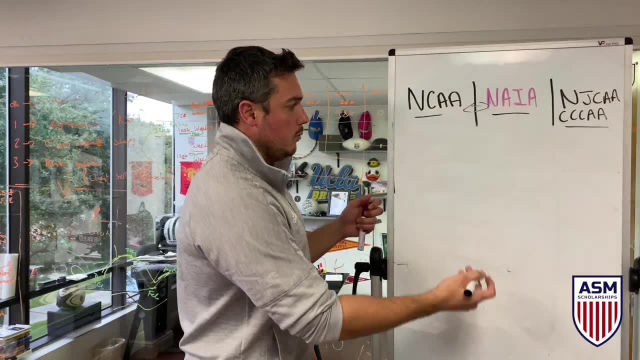 late and you couldn't get into one of these top D1 programs. now how good is the level really per sport? and I kind of mentioned one's really good. but I want to give you kind of like a graph of ideas of like where that really is. 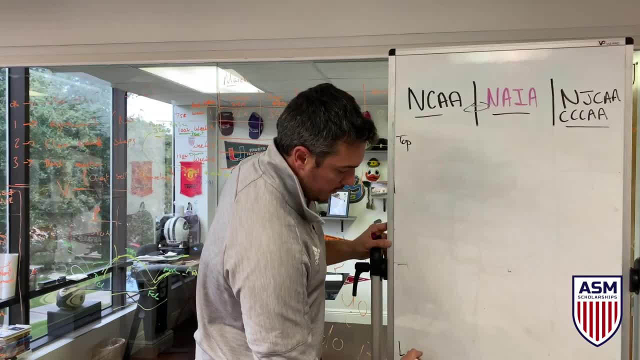 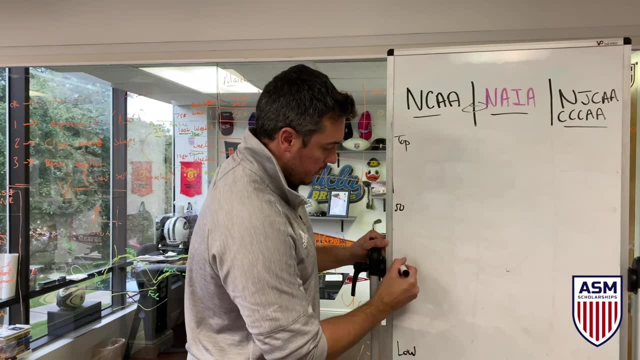 so let's say this is the top level and this is low level. it's not by all means bad, it's just not as good as the top. so let's say this is a top, say 50 programs, top 100, and then obviously what's a 300? 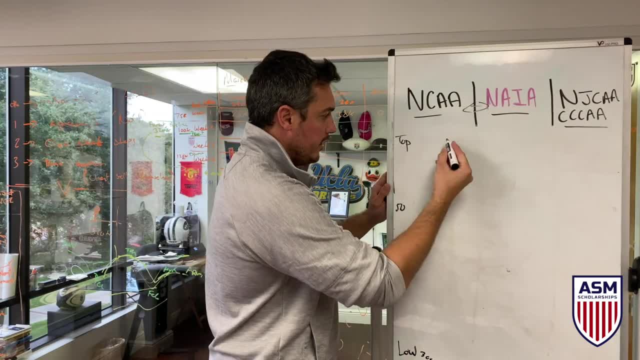 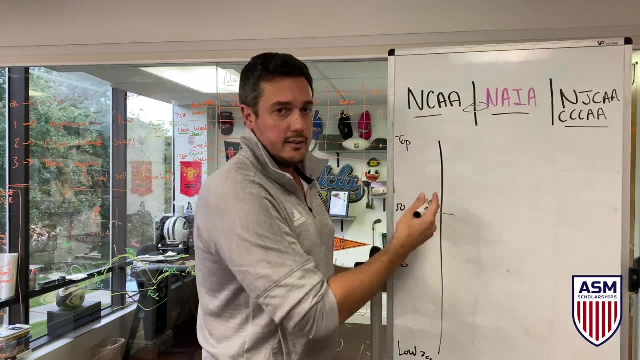 right now, NCMLA will be everywhere from all the way down here. right, we've got good division one programs at the top 50. these are schools like your Stanford's. you've got a lot of good division one programs at the top 50. these are schools like your Stanford's. you've got a lot of good division one programs at the top 50. these are schools like your Stanford's. 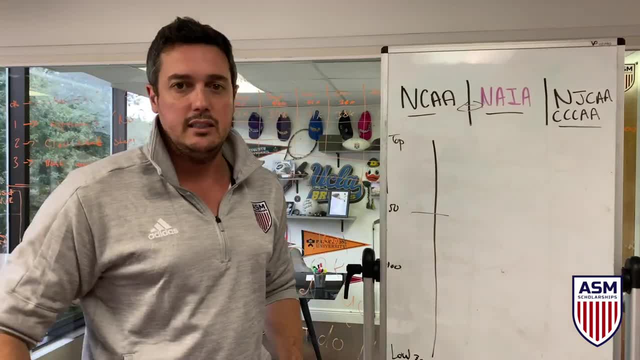 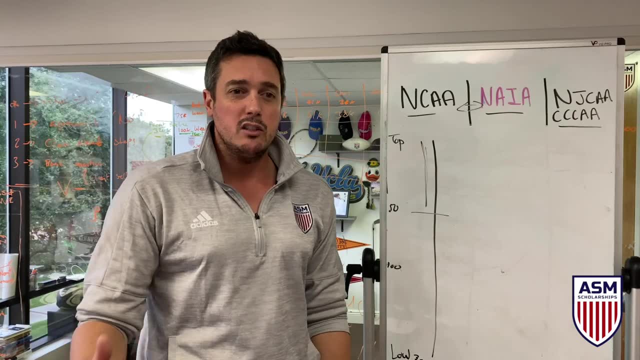 your Dukes, your Vanderbilts, your UCLA's, your USC's, your Alabama's, your Texas A&M's. they're all going to be here. right, these are the. they're always their Clemson's. they're just always been pretty much any sport they do, because they invest a lot of. 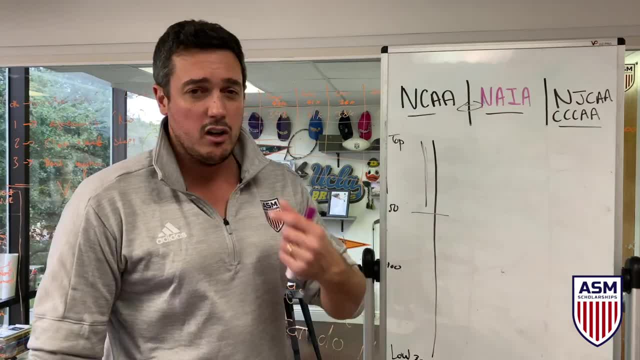 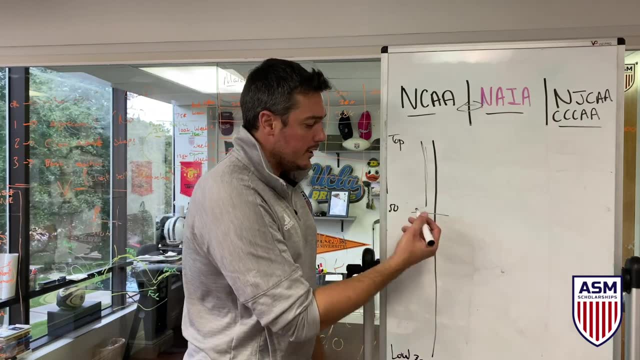 money into their programs and that's how they get more TD rights, more shirt sales, everything. there's like pro soccer football: it's the same thing, but it's college, so they're always have a good. and then you get back the next mix, which tend to be like Colorado State Bowling Green. 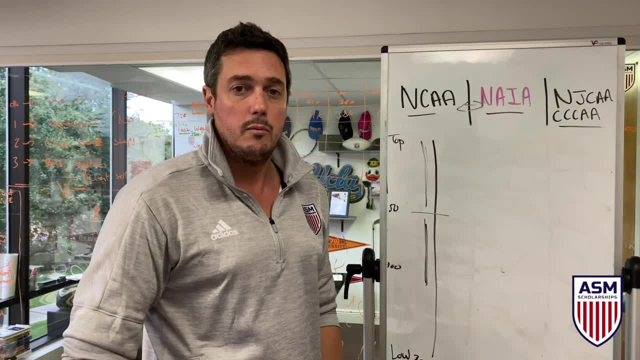 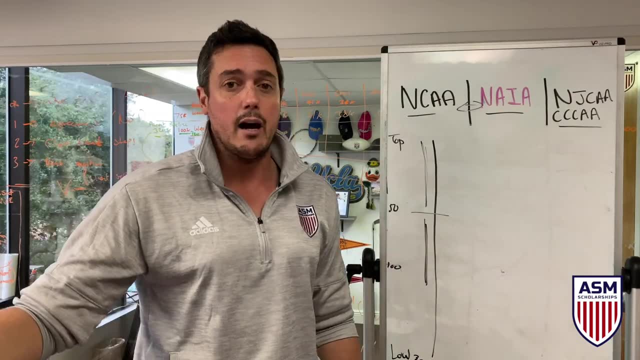 UC Davis still really good Division 1 programs, but they don't, for whatever reason, get into the top 50. Sometimes they do. Colorado State, funnily enough, is actually the golf top five right now, But typically they're like 70th, 80th somewhere around there. And then you get your other university D1s, like Rhode Island, New York. They're like 100 to 300, right, It's like in any sport league: You can start off like 100 and be number one that year, but it's kind of unlikely. 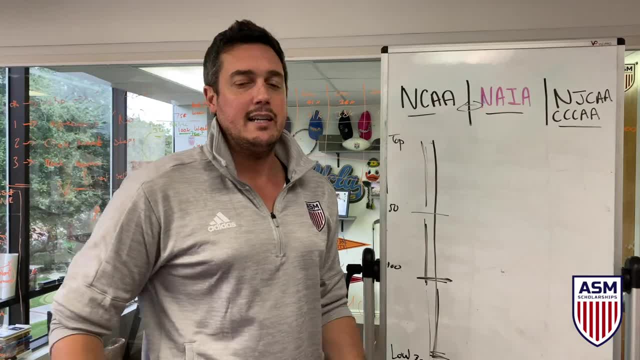 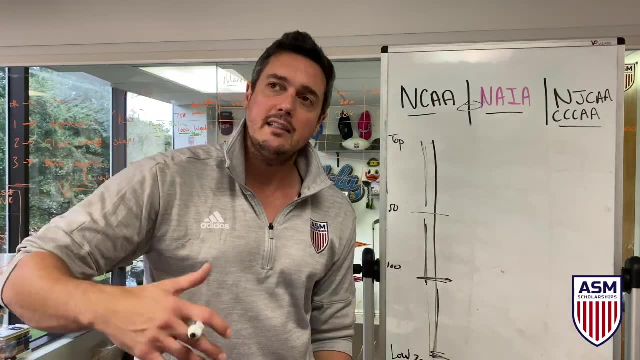 Like normally, these guys are pretty hard to beat. The best way I try and explain this is probably through soccer, the Premier League, just because everyone knows about it, mainly Umancities, your Arsenal, so you know, Umancities Liverpool. 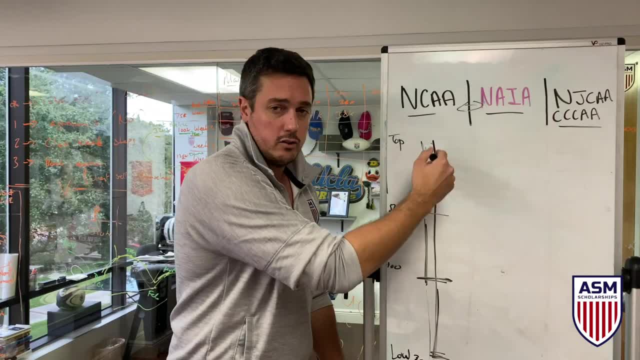 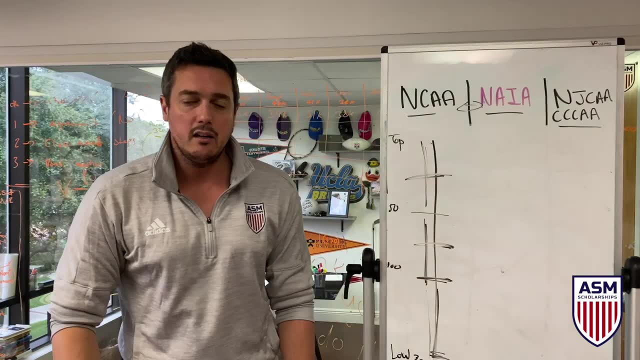 like the last couple of years. they're unbeatable. That would be like the school in the top 50. And then these guys like kind of here to here, say 30s to 70s, they can compete Like Man United. we used to be the best now. 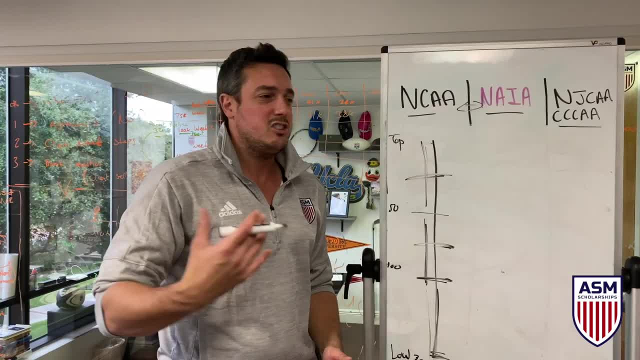 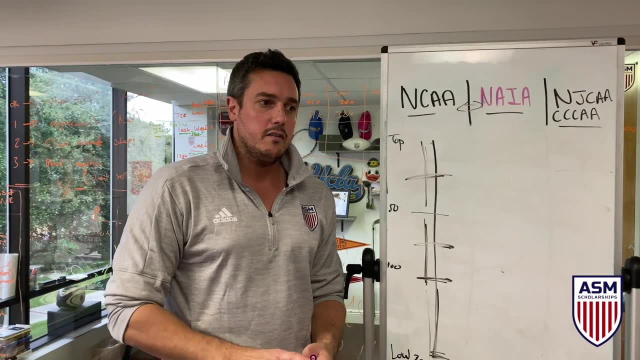 We're not. That's a different story. But we can compete. We're just not challenging for the first top five spots anymore. We're getting there. But also your Chelsea's, your kind of whatever team's- Wolves, maybe They're doing really well. 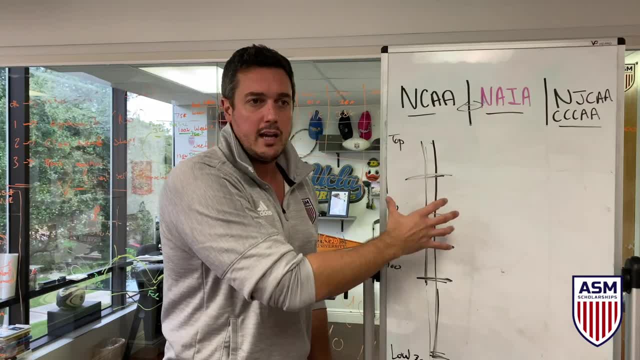 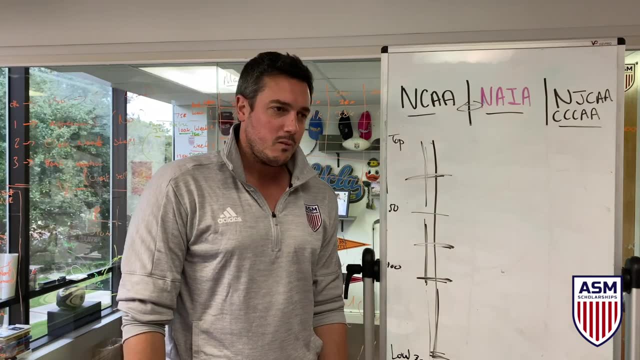 But you get it right. You're not going to maybe be number one, but they're going to be in the top, say the top division area, And then you get your teams down the end which are never really there, like Brighton, or I think West Ham are doing too well right now. 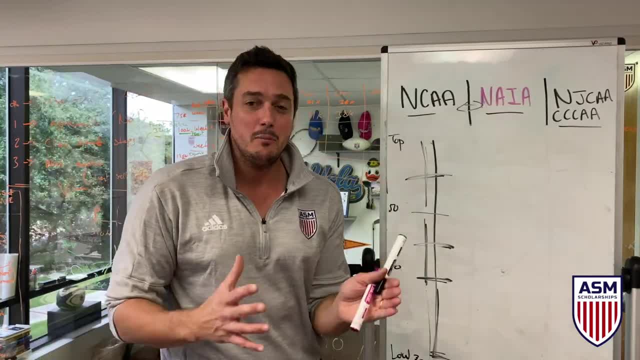 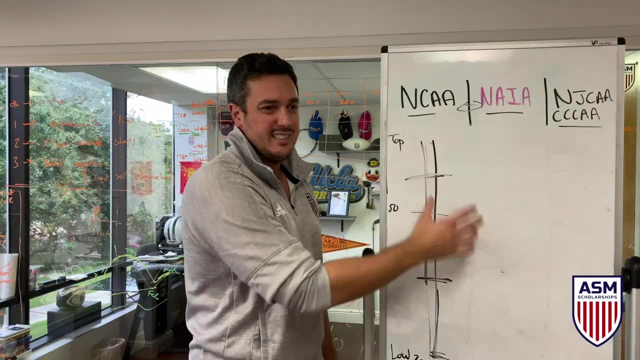 So if you look at any kind of Premier League standard, this is a really funny one to compare it to, but it helps you understand. hopefully, The bottom teams just never really get up there. The middle teams can't compete. The top are always the best. 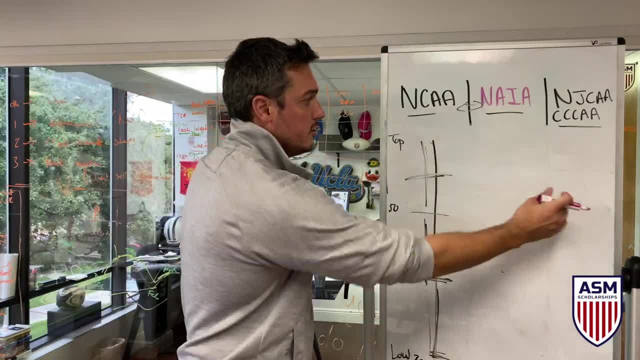 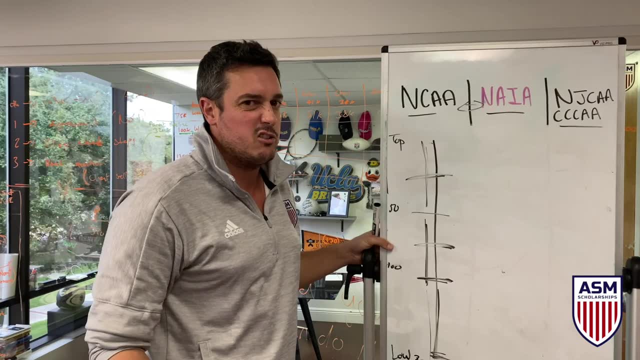 And it's the same here for D1.. Now, what this is going to help you understand is these two NIA, their top teams. now some coaches might get a bit annoyed with me for this, but I think if they're being deep down honest, they agree. 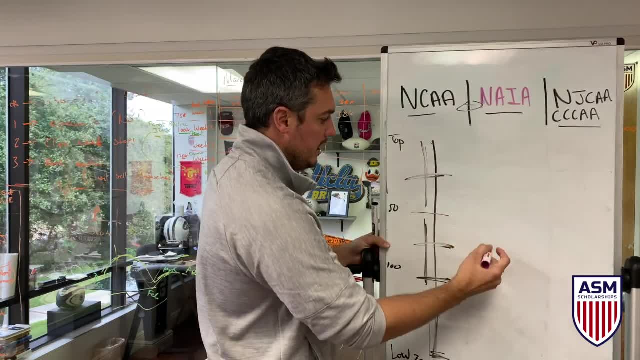 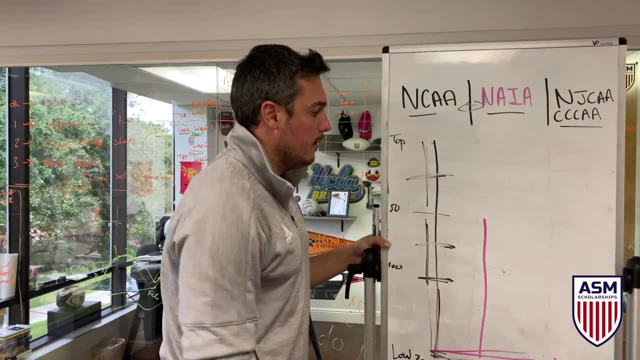 They're never really going to compete at the top, say NIA- They're going to be more like 50 downwards. Everyone's going to end up at the bottom as well, right, Everyone's got teams that don't do so well. They're going to be like 50. So their best say top 20, 50 universities, I'd say would start at 50 top D1 programs. They're more like playing the game of the 50 to 100 level. 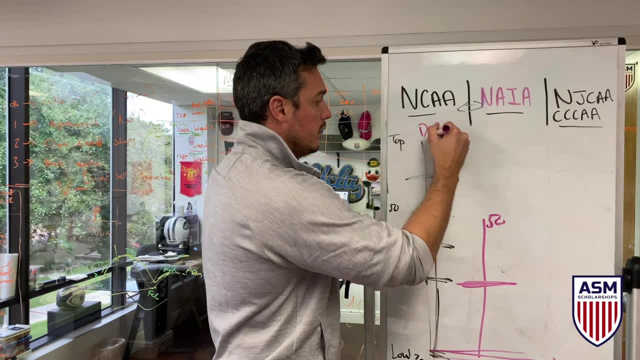 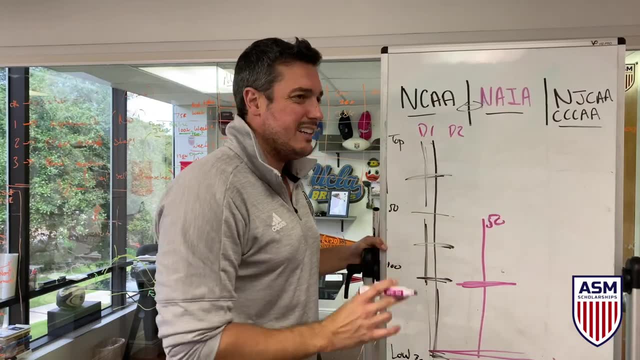 their best programs. Oh, and I forgot to mention D2, so that's D1.. D2 would be now. this is interesting. Their top schools are very, very good. I would again say they're not as good as, say, some of the top D1 programs. 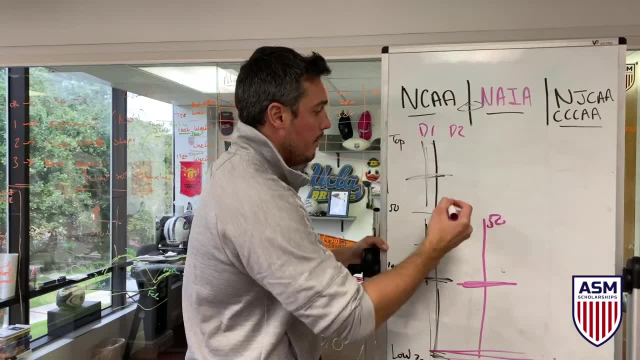 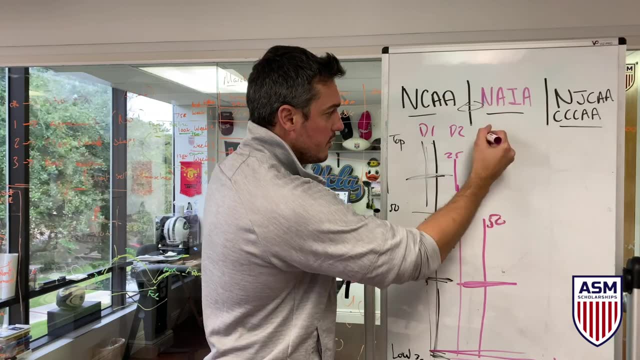 Again, I might annoy some coaches there, but it is real what it is. They are better than this. I'd say D2 is kind of like here, like 25, right, And it goes down like that. D3, I'm going to say that's a little bit. 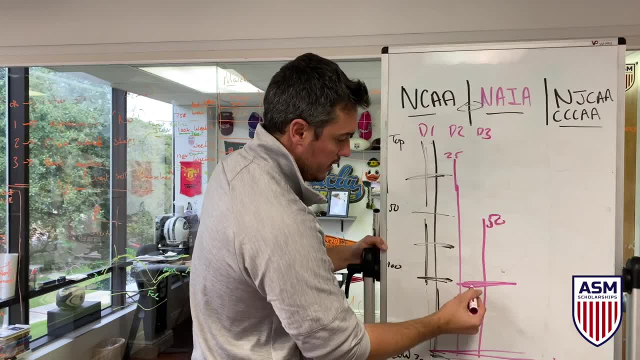 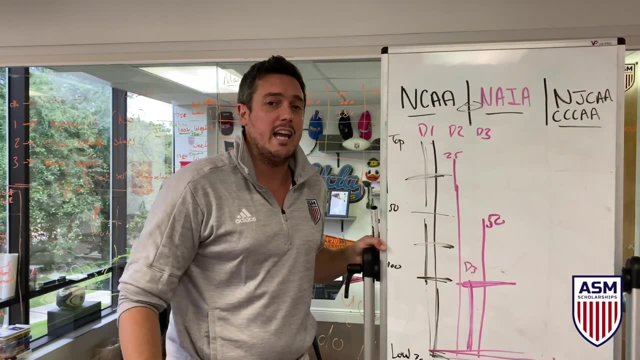 a little bit different. a lot different, I'm going to say. they start kind of at 100, 100 and down right, So that's D3. Because they're not really competitive. They are competitive but they're not the same level as a D1, D2.. 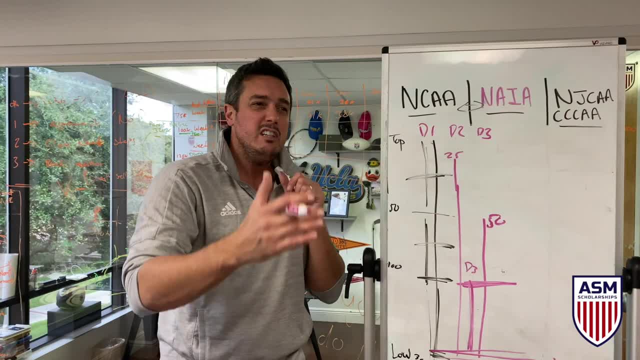 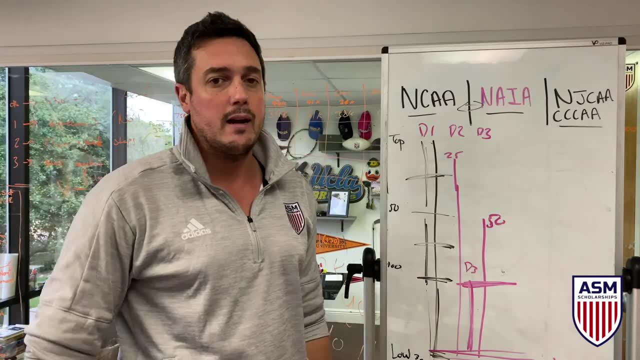 A D2, any top school is just as good as the most top D1s, but the really, really top D1s are like in whatever sport they're focusing on, they're just like another level And if you go visit those programs, you'll see it. 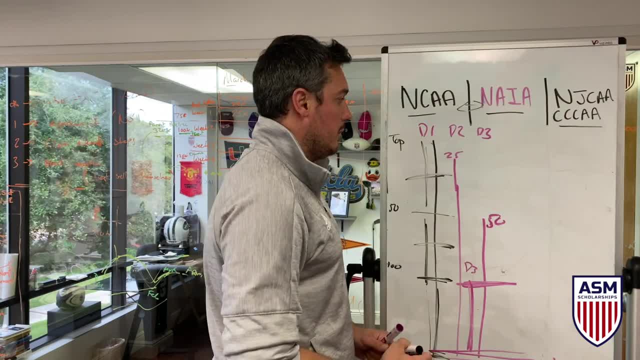 Now the NJCWM. this is a lot different in my opinion- Yeah, In my opinion, but I've done this for 10 years. it's basically what I've seen. I would say they're the same as D2.. 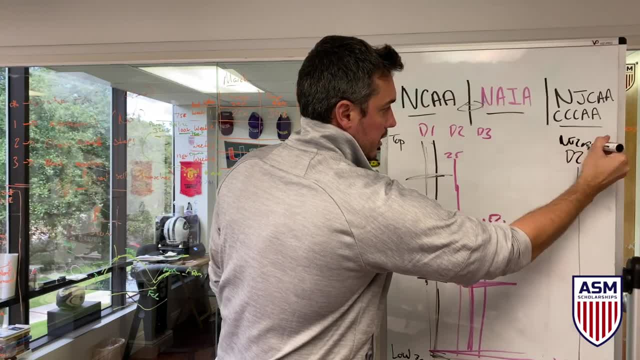 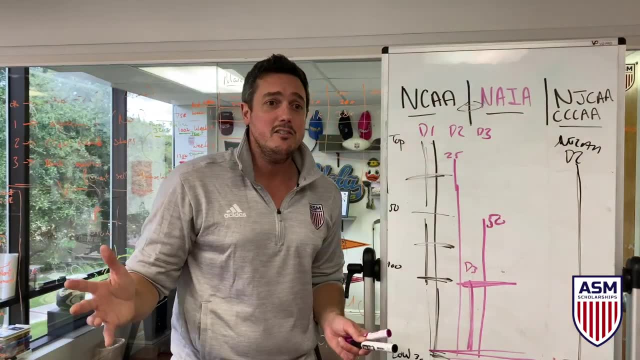 I would say they're the same as a D2 level for an NJCWM, Because their top programs would be most even D1 or D2 programs. I know this because I played junior college for one year in Iowa, So I play at this level and I play at the other level. 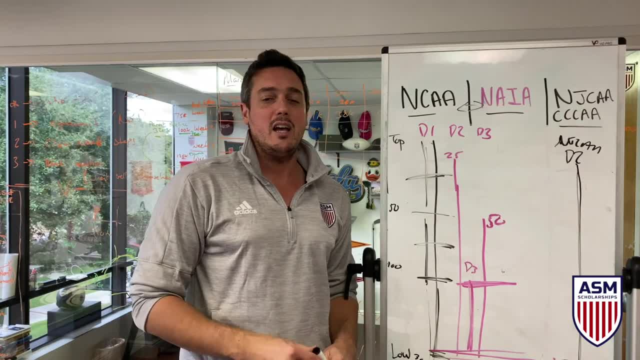 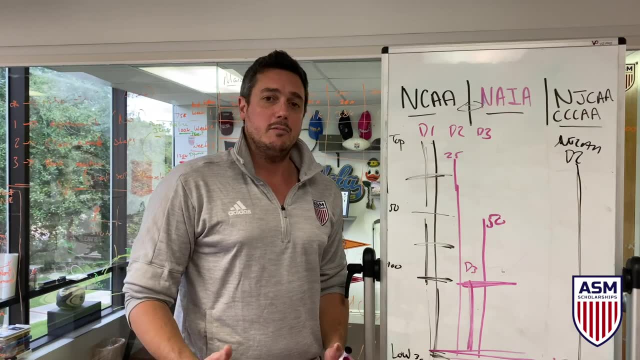 so I know the differences And I know we had one of the best golf teams at junior college. We beat D1 programs. We had like imitations we went to We would beat them. So I know it's possible And I know basketball teams are the same thing. They beat D1 programs, They beat D2 programs in invitational tournaments. So they aren't just as good at the top level. But it's like anything At the bottom level, any division, they're just the same as everybody else. 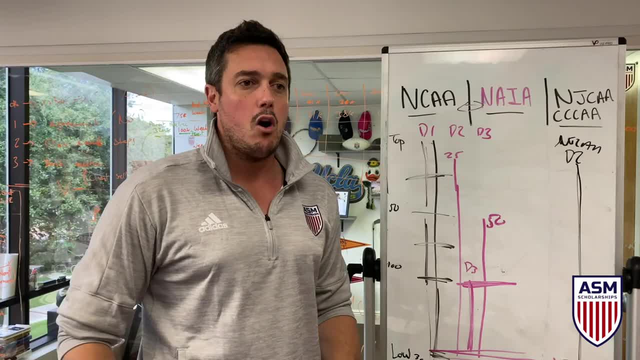 So you've got to think again. why are you doing this? If you're doing this to be a pro athlete, your goal would be to probably get here eventually. Now, if you don't get in, don't be upset yourself and quit. 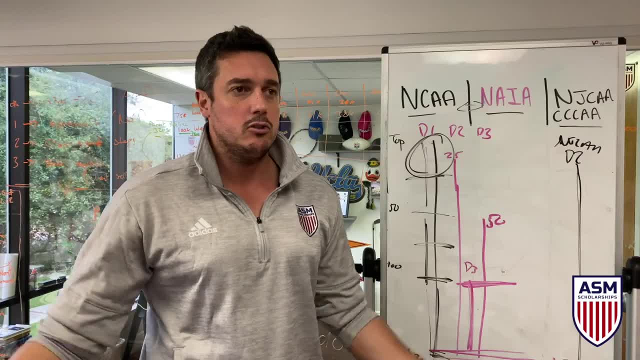 That's not the way you're going to do it. It's like saying: I want to play for Manchester United, but I'm just not good enough. Yeah, you've got to work yourself up the process. You might need to start at a D2 program. Maybe you start at a 100-rank D2 program And then you transfer two years later. Maybe you start at JC, Maybe you start like around here and you transfer later. The key is get yourself your name out there in the competitions. in the US system, preferably than playing overseas. as fast as you can when you're 18.. And then, if you're good, you will be transferred. There's no doubt about it. If you're a good player, these top programs will come knocking into you. 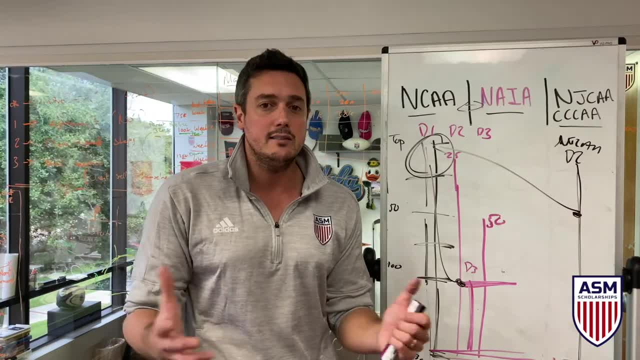 especially if we're helping you. They'll come knocking on your door and you'll get in Now. if you're good at 16,, 15,, we'll make that happen sooner. You'll still come at 18,, but you'll commit sooner. 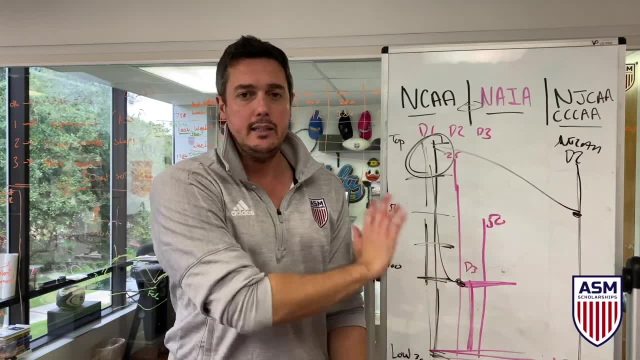 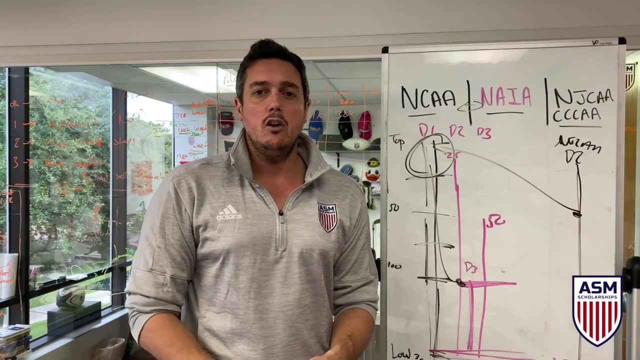 Okay, Now that's just for the sport level. Academically, completely different. This is just the sport level rankings. Academically, it's super easy. I'd go to like a Forbescom New York Times- look at the academic rankings. 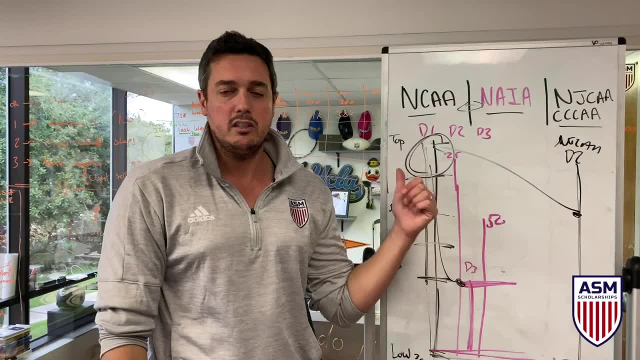 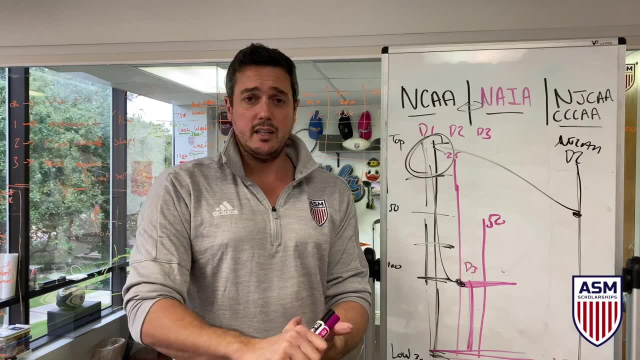 That gives you like a Division III school sometimes are better than most D1 programs. when it comes to academics, It depends on the school. So you've got to research what academics you want to do. what do you want to study? where are the rankings?